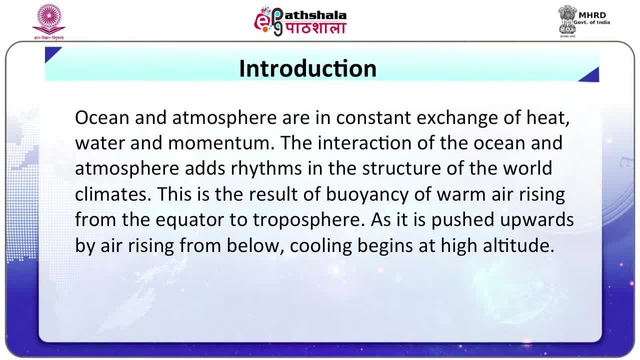 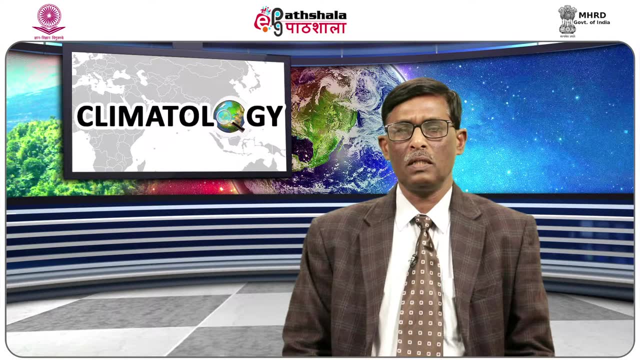 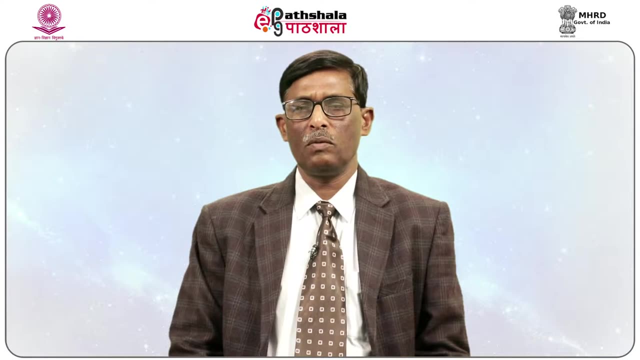 exchange of heat, water and turbulence. The interaction of the ocean and atmosphere geography. The interaction of the ocean and atmosphere adds rhythm in the structure of the world climates. The oceanic interaction transports moisture in atmosphere in the form of water vapor. Solar radiation is the ultimate driving force for all motions in the ocean. 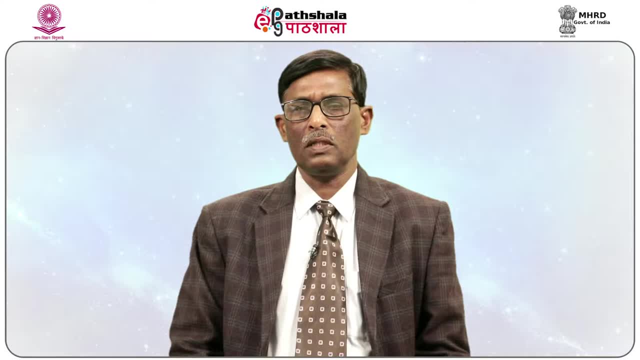 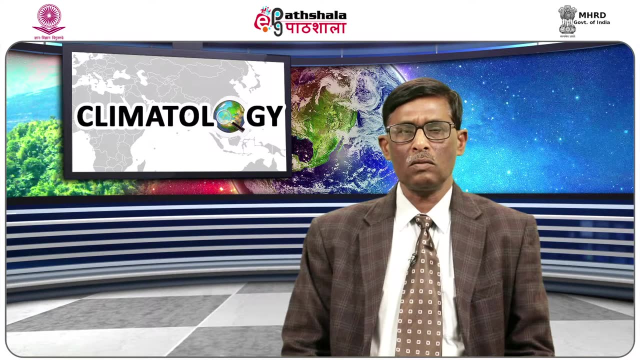 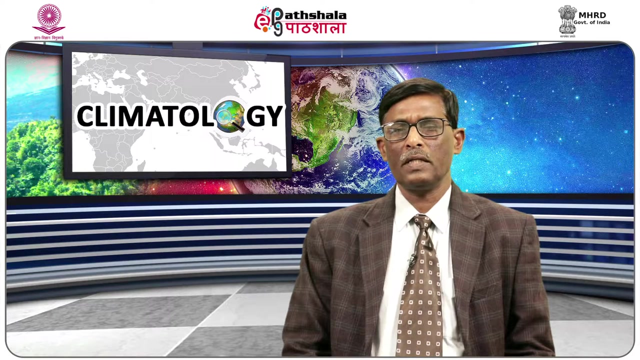 and atmosphere and gives rise to the pronounced and regular diurnal and seasonal cycles throughout the world, Climate not only displays repeating and regular cycles of solar radiation, but also displays variability that is not correlated with solar radiation. An attempt has been made to study the ocean and atmosphere interaction and its resultant outcomes in this module. 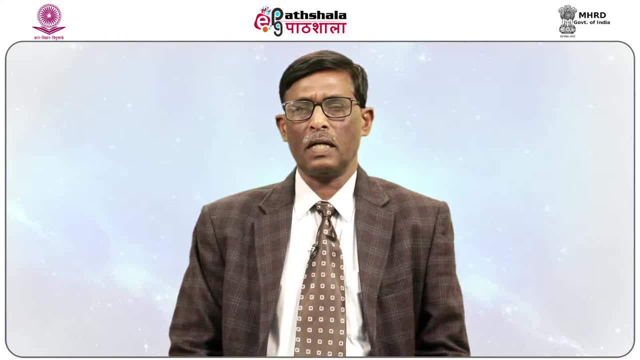 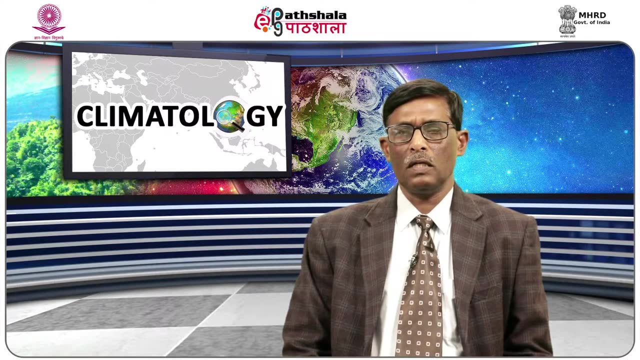 Forces responsible for ocean atmosphere interaction. The motions of the earth with reference to sun are responsible for the generation of energy and its distribution in different parts of the earth. Earth's rotation results in causing day and night. The variation in the length of day results in the receipt of solar. 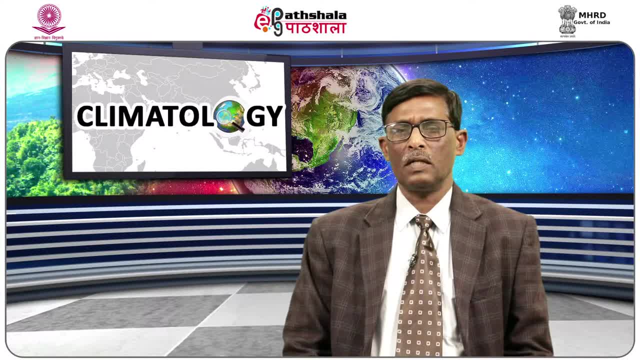 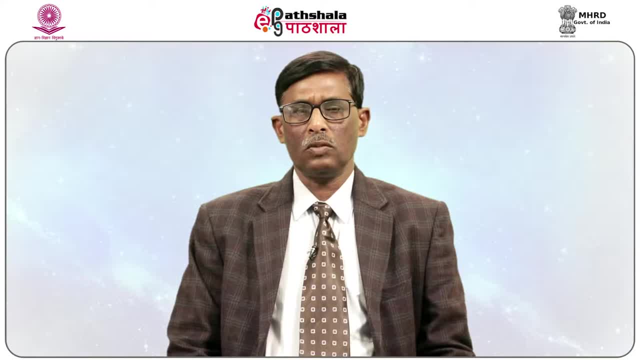 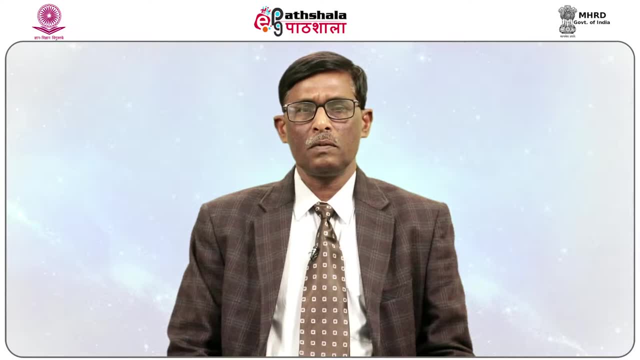 energy, its absorption and transmission. Earth's revolution results in the creation of new life forms. Israel's moral physician of the theorticology has found, through the also gladiatorial project, that specific properties of the Earth, such as feed, load naszymal abuse. 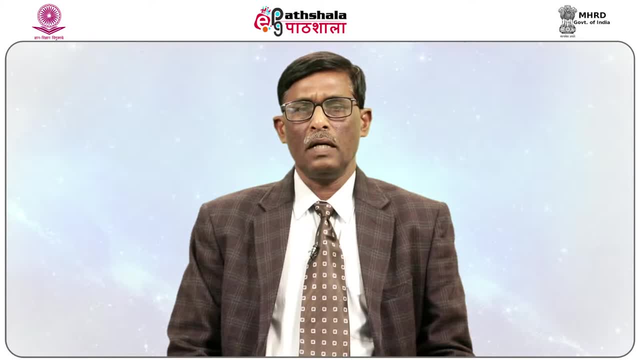 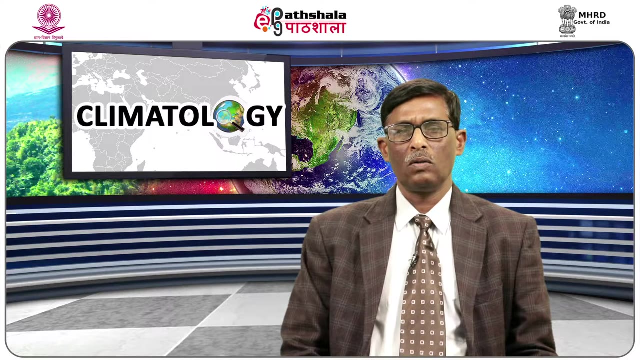 of the environment and outside influences can will be at one timerupal to have a messy covert�arless. Letís now look at the natural process in the oceanic atmosphere í for ocean-atmosphere interaction, There are several processes, such as radiation conduction. and convection that are responsible for the transfer of energy from source. Similarly, energy transferred is subjected to several other processes that interfere and modify the impacts In terms of factors such as winds, waves, currents and air are responsible for interaction between ocean and atmosphere. Medium of interaction: The energy received. 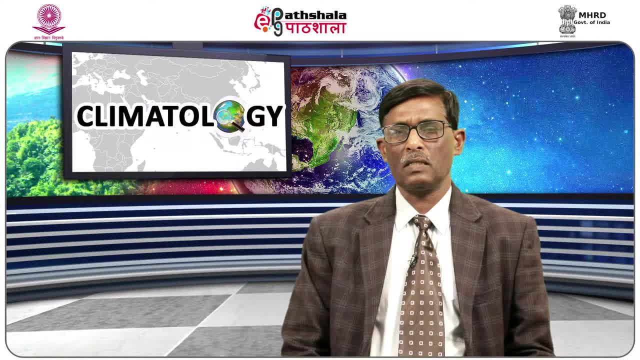 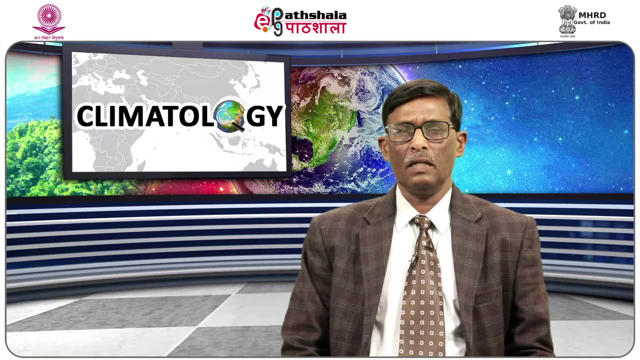 from the sun is in a systematic circulatory pattern. It is from sun to earth surface, that is, land and water, Water surface from land and oceanic surface at atmosphere and return flow from the atmosphere to land and ocean surfaces. The cycle of interaction is augmented by processes such as radiation. 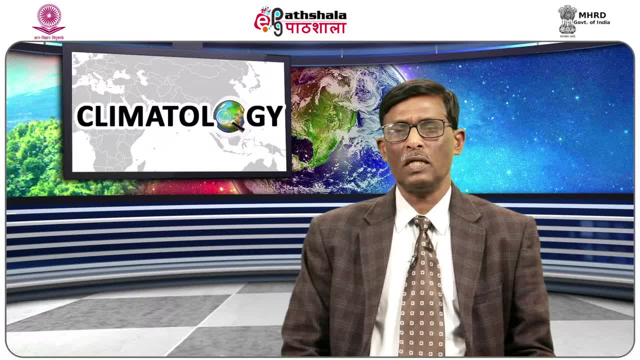 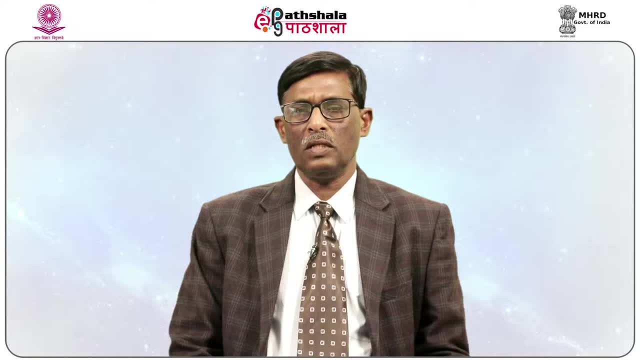 conduction and convection. The energy so transferred is subjected to modification by the processes such as reflection, refraction and reradiation. Air and the ocean are continuously exchanging heat. As the ocean has a higher heat capacity, it takes longer to adjust to changes in coming radiation and therefore tends to change the temperature slower. This means that the surface of the sea is usually a different temperature at the air immediately above it, and heat is transferred between ocean and the atmosphere. Winds- The movement of wind from ocean to land is an important factor in transferring the moisture towards land areas. There is a marked difference between the response of a large land mass and oceanic surfaces to heat received from the sun. During summer, the wind over continents is much warmer and less dense compared to the oceans. Most of the solar energy received at the ground by the continent is confined to a thin layer. 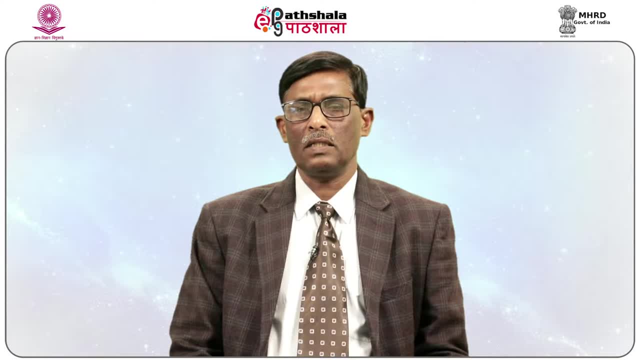 of the earth. More and more solar energy received on the land surface is used in heating the nearby air parcel. On the other hand, solar energy is able to penetrate much greater depth of the oceans because of the atmosphere. The nostroids are observed as numerous over the entire Her לקroid Bartlewice region. 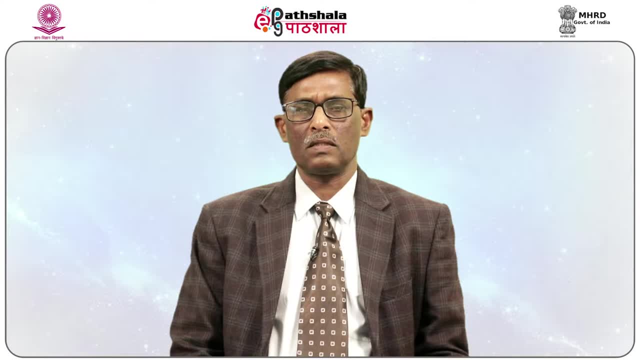 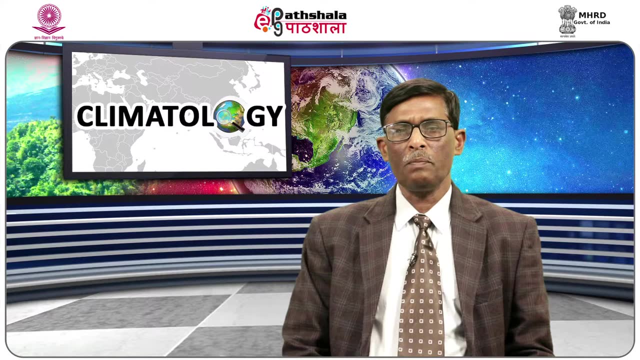 the interest in the ocean is high. The current moment values are found to adjust to some more than half the current. with respect to solar energy allotted to an thankful, connectionriois environment and continually sparking light for solar energy in light of a given climate, somewhat sourced, pinned to the 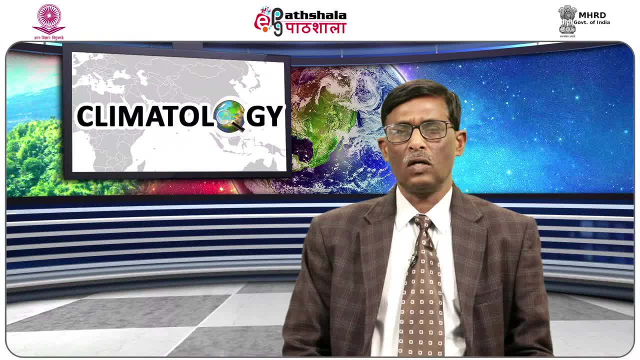 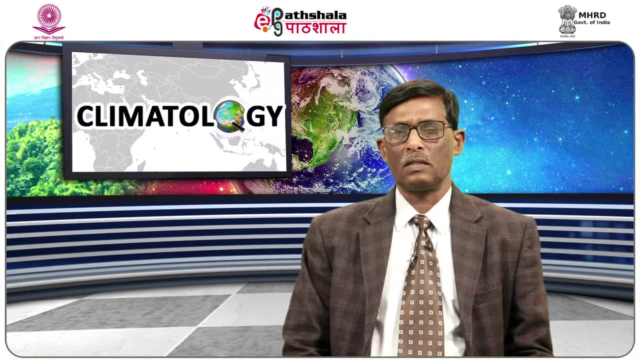 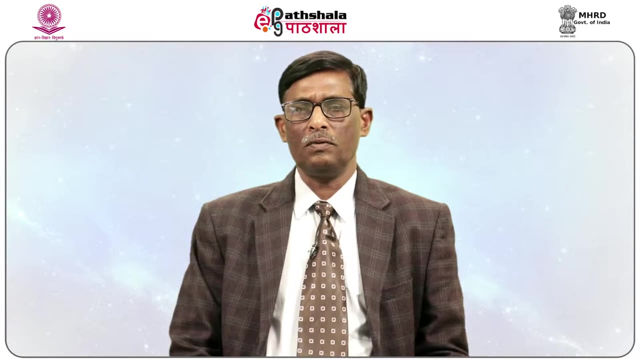 students their winds. brother I �� how did I say What What the rise in temperature during summer is much less over the oceans than over the continents. Now let us see about the salt and aerosols. Meteorologists are of the opinion that very large quantity of salt particles in the form 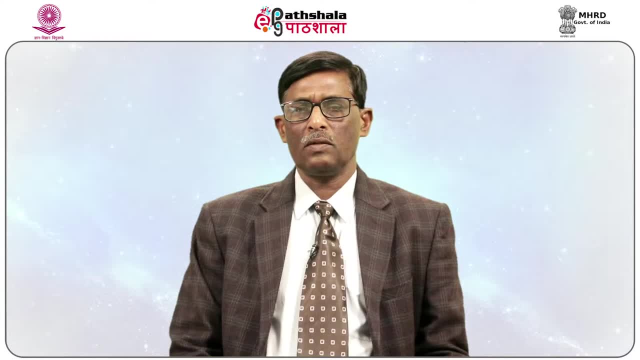 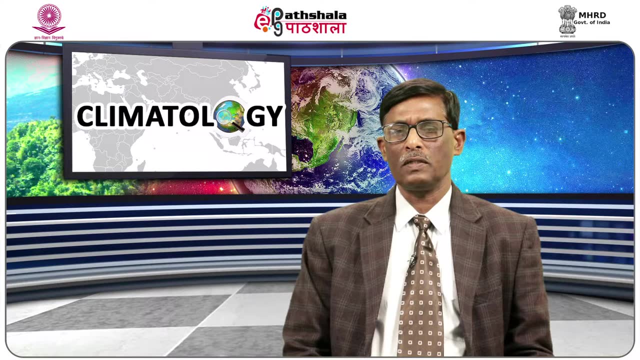 of aerosols are injected into the atmosphere by the breaking of sea waves. When waves strike the coastal region of the large land masses, they release a large volume of spray. Millions of minute salt particles are injected into the free atmosphere in this manner and they act as a storehouse of nuclei for condensation. Salt is continuously brought. 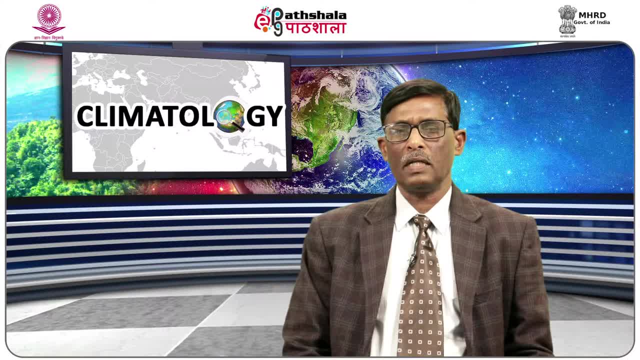 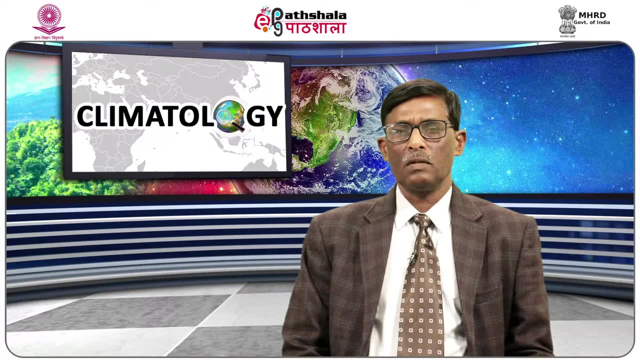 into the ocean by the waves. The salt particles, then, are absorbed by the sea waves by draining off the continents. They carry minerals by dissolving from the rocks and run over and deposit the same in the ocean floor. Water evaporating or freezing at the ocean surface leaves the remaining water saltier. 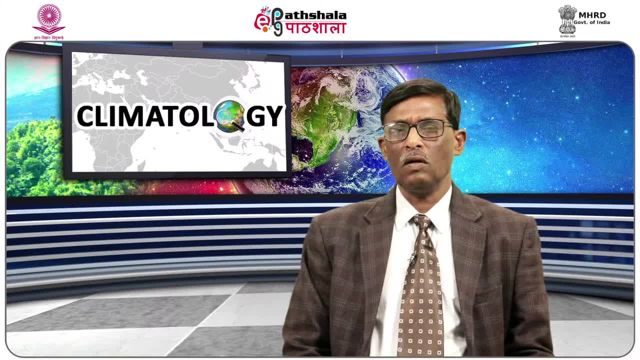 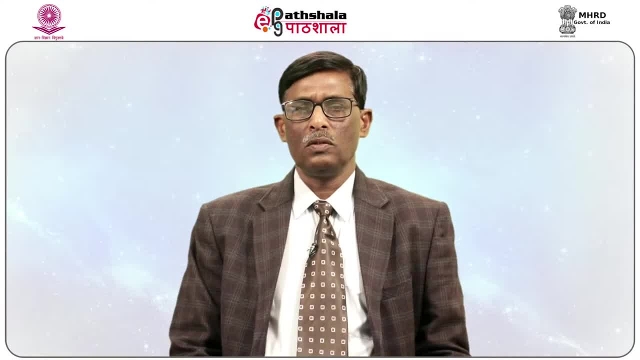 But rain which is not salty dilutes the salt content of the sea concentration of the ocean. Now coming to feedback mechanism, There are many feedback mechanism between the oceans and the atmospheres. For example, evaporating water can condense in the atmosphere to form clouds. These reflect both incoming and outgoing radiation. It is 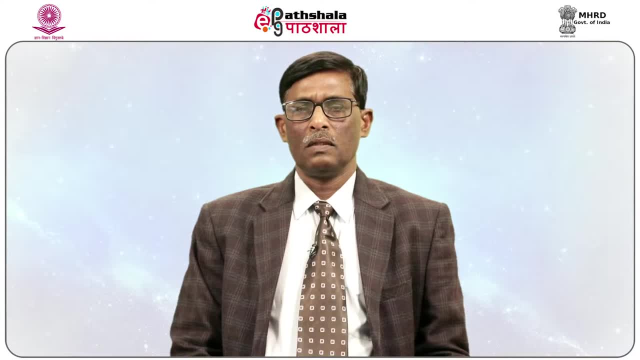 because of this mechanism that cloudy nights are warmer than the clear ones. The system thus determines the temperature of the ocean surface. Surface air and air aloft are in opposite motion and thus form a cycle. It helps in transferring heat and other objects to upper surface. 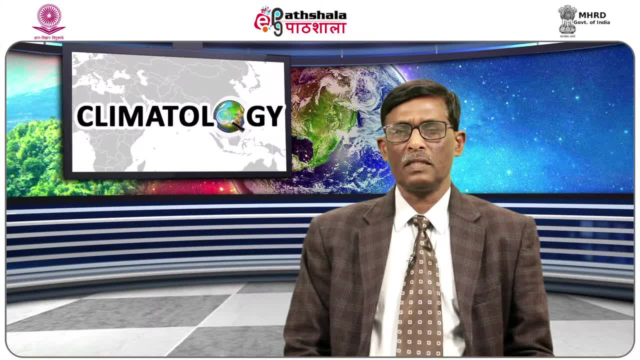 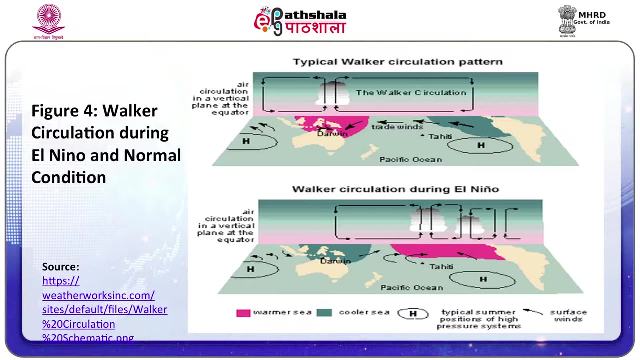 The most famous among such climate variations is the Atmosphere Southern Oscillation, which we call Walker Circulation, which was put forward by Walker in 1924, and its oceanic counterpart, that is El Nino. Let us talk about Walker Circulation, The interaction between oceanic water and atmospheric 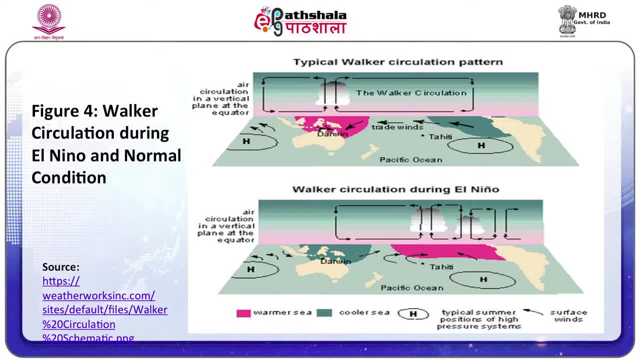 winds are closely related. Sir Gilbert Walker was the head of the Indian Meteorological Service during 1904 to 1921.. Based on observation and experiments during the course of his assignment, Sir Gilbert Walker has developed a conceptual model of air circulation in the tropics in. 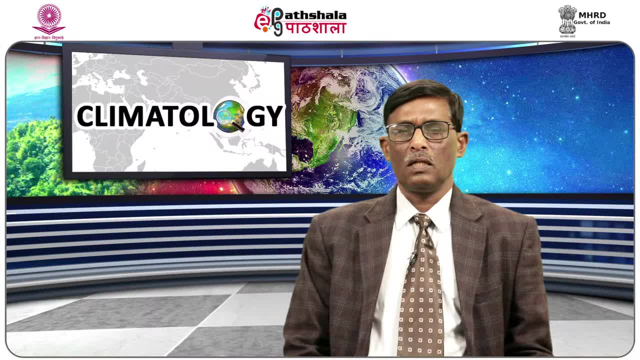 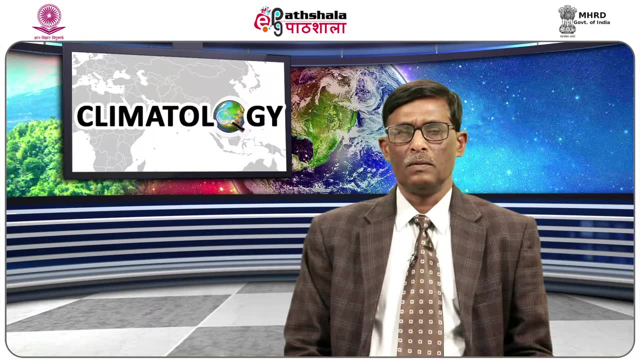 lower troposphere, According to the model parcel of air, follow a closed circulation in the zonal and vertical directions. Walker circulation is also known as Walker sail. It is the result of a difference in surface air pressure and temperature over western and eastern Pacific Ocean: A pressure gradient. 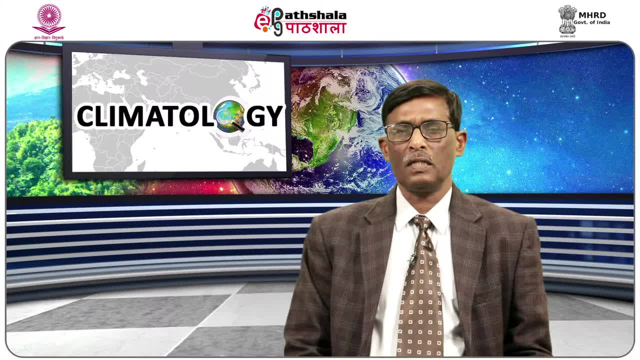 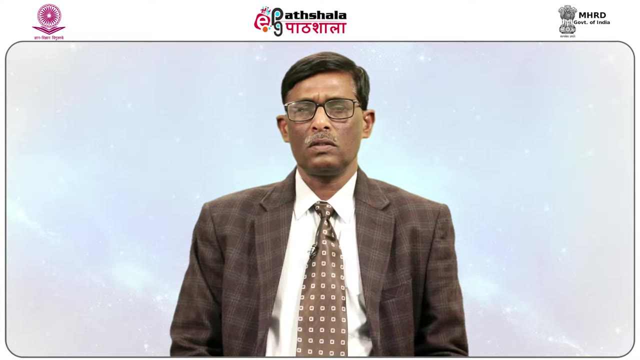 from east to west causes surface air to form: high pressure in eastern pacific to low pressure in western pacific. A line differentiating cold water layer with warm water layer is known as thermocline, The rising branch of pacific shell of walker. circulation follows. 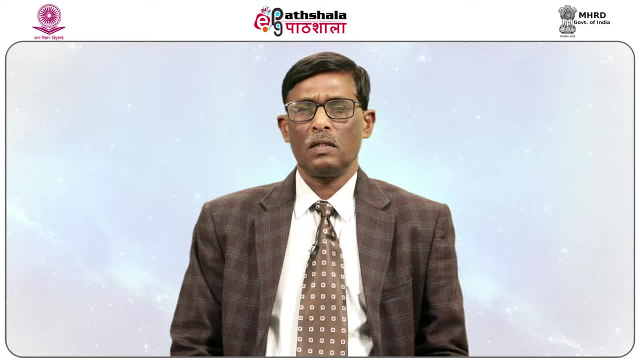 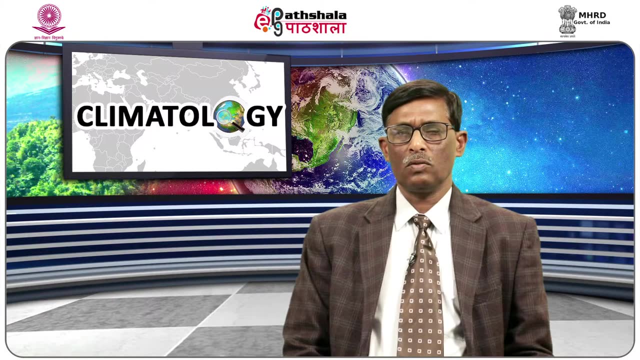 this warm pool which moves eastward. Sir walker discovered a significant relation between monsoon rain over Indian peninsula and south American pressure in April-May. He opined that overall effect of energy received from the sun was to set up impulses of the energy for natural oscillation in atmosphere. Accordingly, eastern pacific ocean remains cooler with high 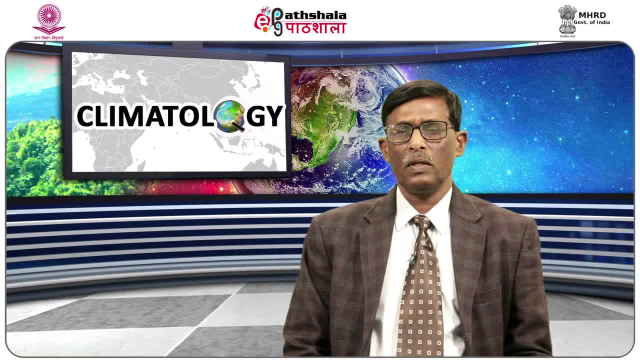 air pressure. The surface winds blow in east-west direction, while winds aloft move in west-east direction, thus completing the circulation cycle. On the contrary, the western pacific ocean becomes cool and the air becomes cool. 3. What is the effect of green light on the earth? 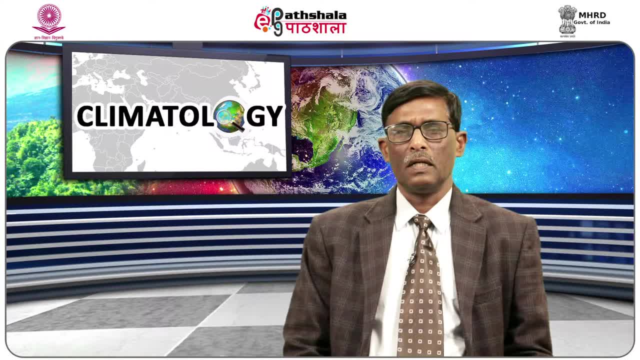 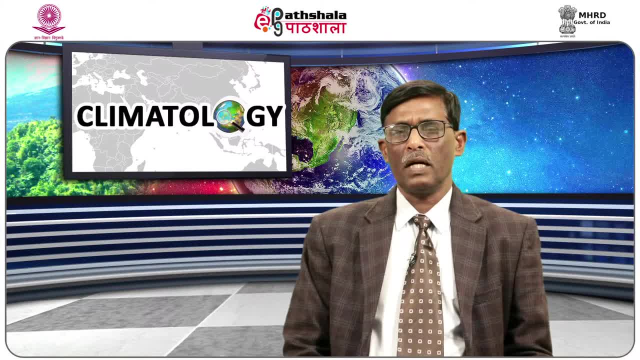 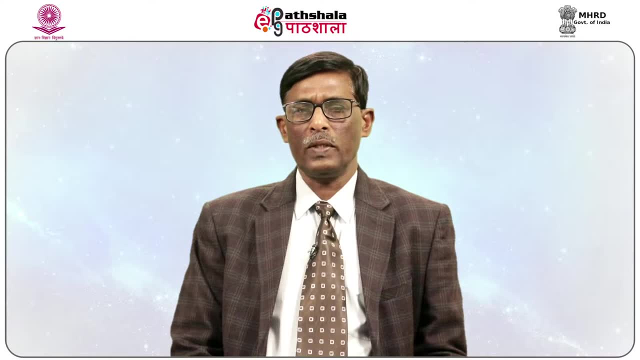 the same time, the eastern pacific becomes warmer and the air over the area is lighter, and hence a low pressure is result. Thus, the winds are west to east on the surface and east to west in the upper air motion. Such a situation is known as El Nino, which is responsible for a weak summer monsoon in 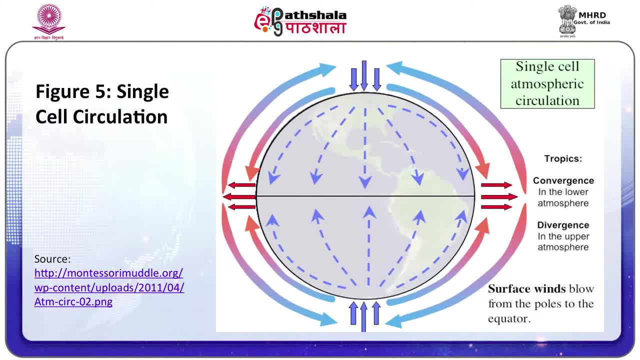 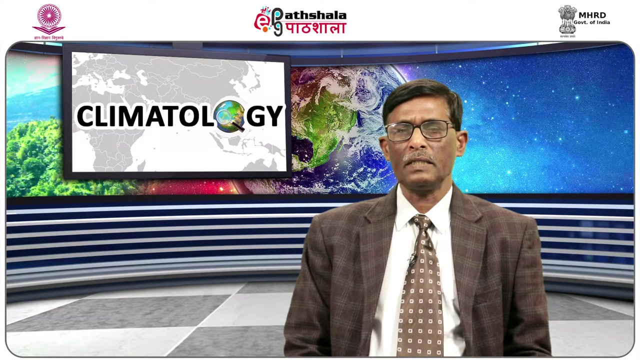 the northern hemisphere, Now coming to the atmospheric cell in ocean atmosphere interaction. Because of rotation and differential heating of the surface of the earth, air motion takes the form of cells. The air motion of the cells on the ground is opposed to the air motion aloft. as it completes the cycle, The operating cells from equator to pole are: 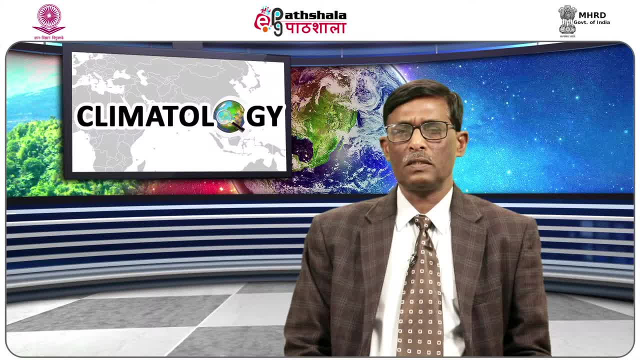 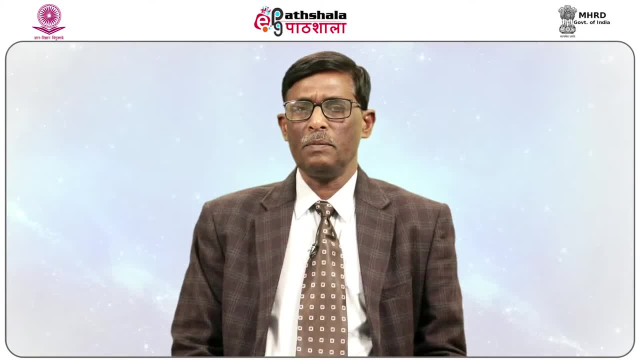 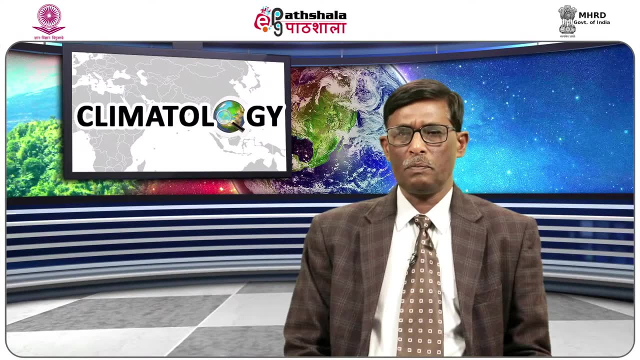 three. A brief account of these cells and their role in ocean atmospheric interaction is well explained. It is named after George Hadley, which was invented by him in 1735.. There is primary circulation cell, known as Hadley cell, and two secondary circulation. 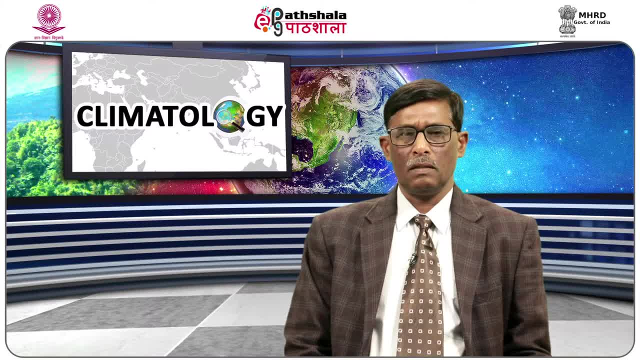 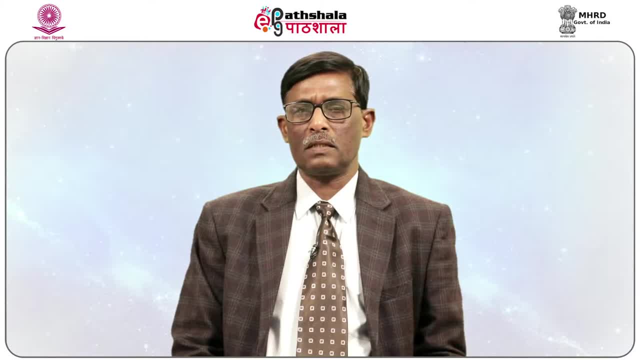 cells at higher latitudes, known as ferral cell and polar cell. Hadley cell suggested that the distribution of solar heating would lead to rising motion in the equatorial regions and sinking motion near the poles To compensate for the upper flow from the equator to pole. Hadley envisaged a return flow from pole to equatorial region. The distribution of solar the equator at lower latitudes. It can consist from 30 to 40 degrees north and south and is mainly responsible for the weather in the equatorial regions of the world. 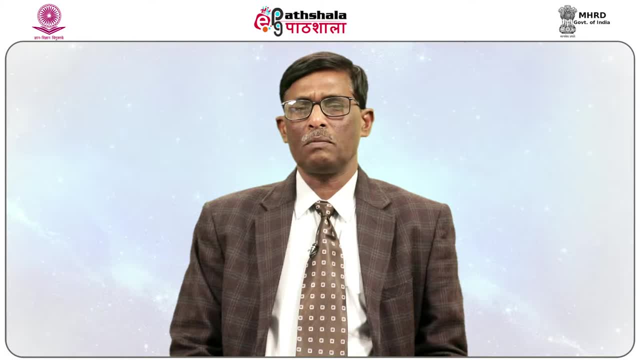 The Hadley cell is a tropical atmospheric circulation that features air rising near the equator, flowing poleward at 10 to 15 kilometer above the surface, descending in the subtropics and then flowing equatorward near the surface. The circulation creates the 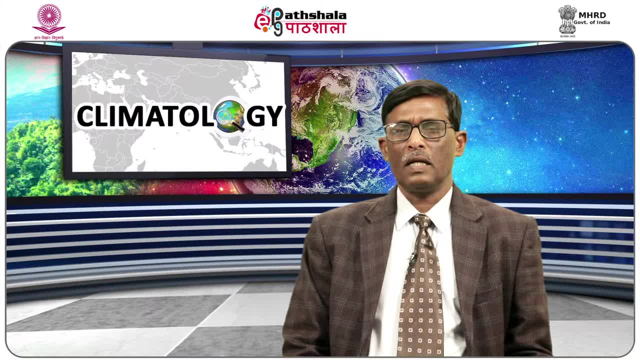 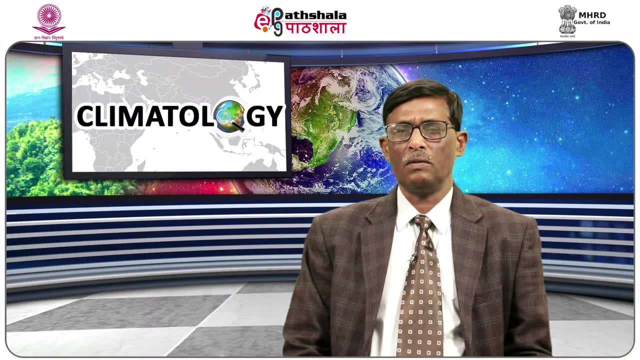 trade, wind, tropical rain belts and hurricanes, subtropical deserts and the jet streams. Now, coming to the Farrell cell, William Farrell, in 1856, has pointed out the effect of Earth's rotation, or the Coriolis force, on large-scale movement of air. Farrell has pointed out that Hadley's model 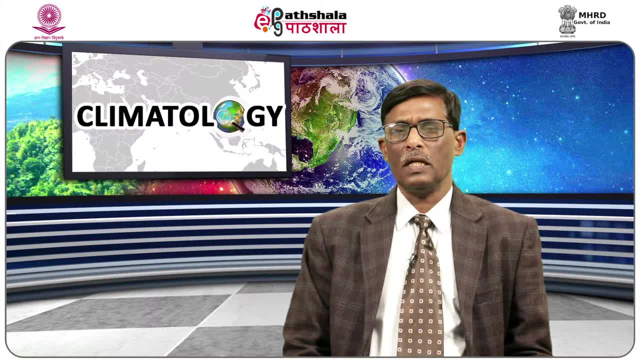 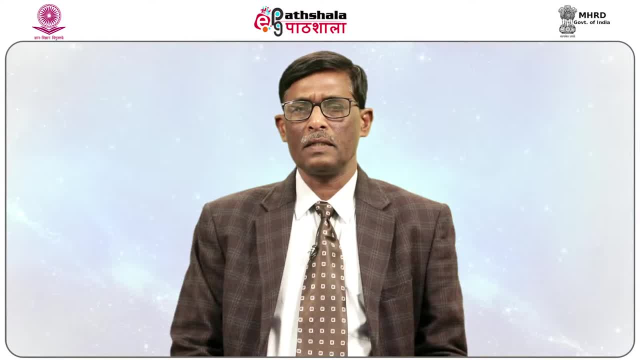 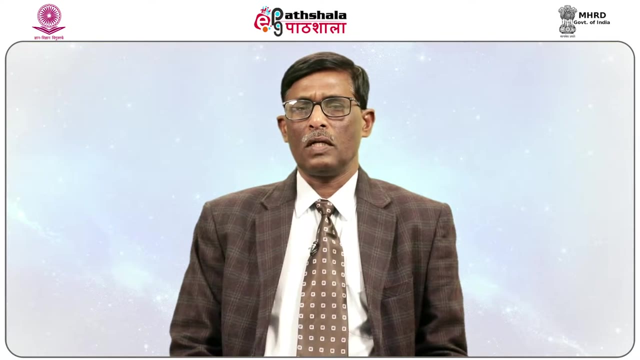 does not take into account the relative loss of heat from upper layer of the atmosphere. He has explained that towards higher latitudes a loss of energy by long wave radiation exceeds incoming solar energy from the sun. The loss is equivalent to a cooling of the atmosphere by about 1 to 2 degrees Celsius per day. There is then 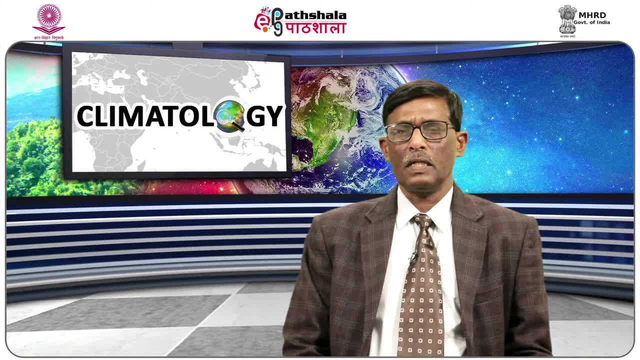 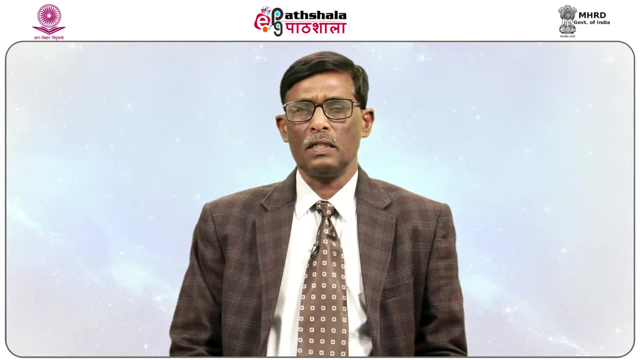 Then a middle cell between 30 degree north latitude to 60 degree north latitude in which there are westerly winds at the earth's surface and easterly winds aloft. This is known as feral cell. The location of tropopause in the cell region is about 10 kilometer above the surface. 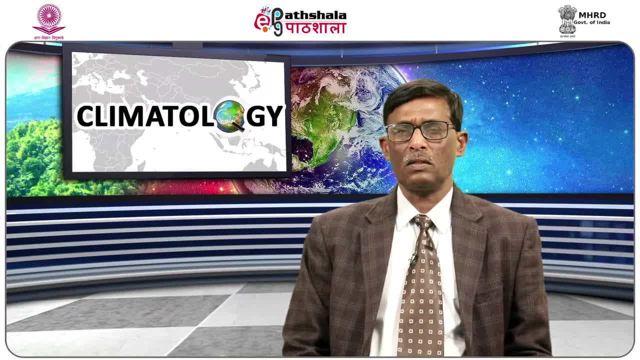 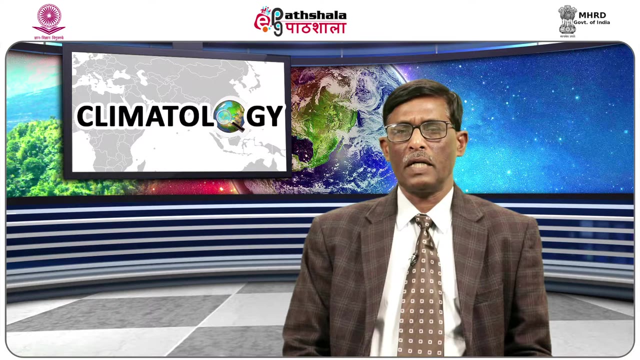 Now coming to polar cell. Between 60 degree north and the pole, there lies a polar cell. The surface winds in this case are easterly and the upper winds are from a westerly direction. The polar tropopause is located at about 8 kilometer above the surface. 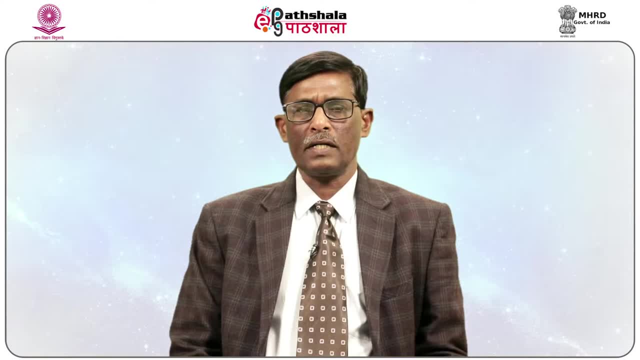 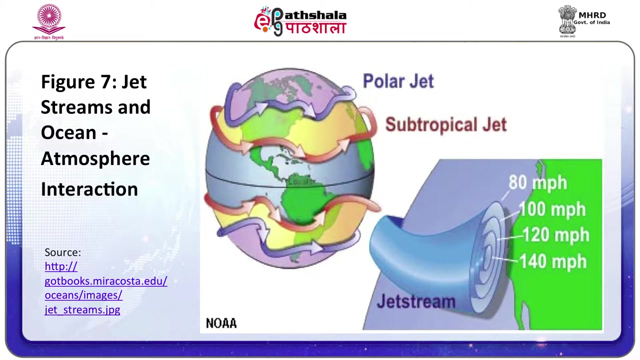 Thus the effect of heating And convective currents is dominant in tropics, while cooling and subsiding currents dominates towards polar areas. Feral cell is significant as it balances the two opposite systems of the air circulation. Let us discuss about jet stream in ocean. atmospheric interaction. 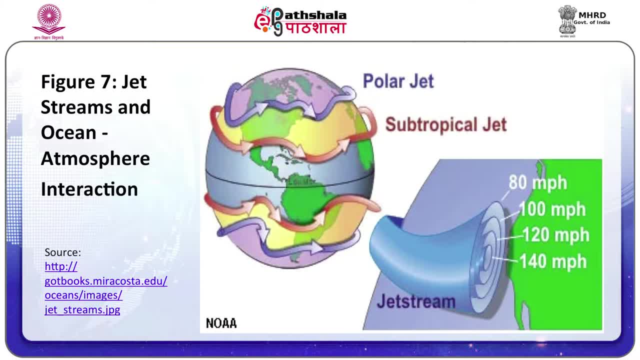 These are narrow, meandering upper airs. High speed winds. High speed winds- They play a decisive role in accelerating the dynamic situation- that are conducive to transfer of energy and moisture to the atmosphere. A brief account of polar and subtropical jet is explained below. 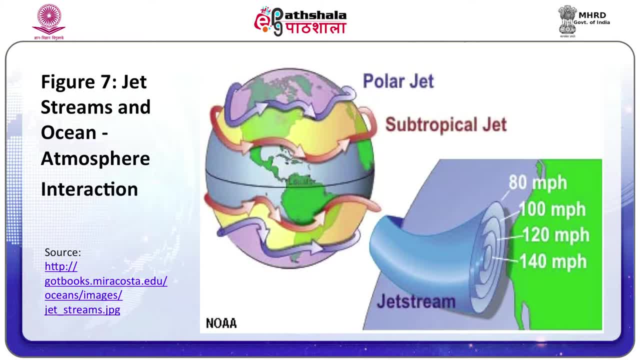 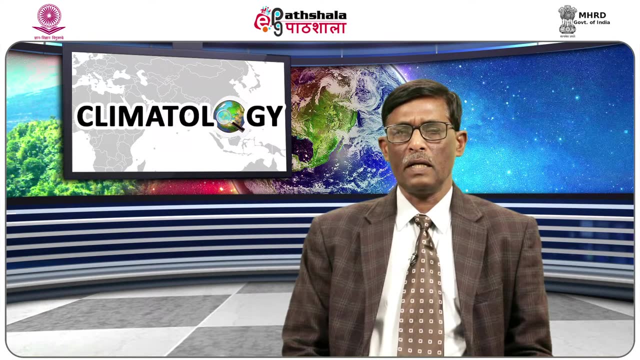 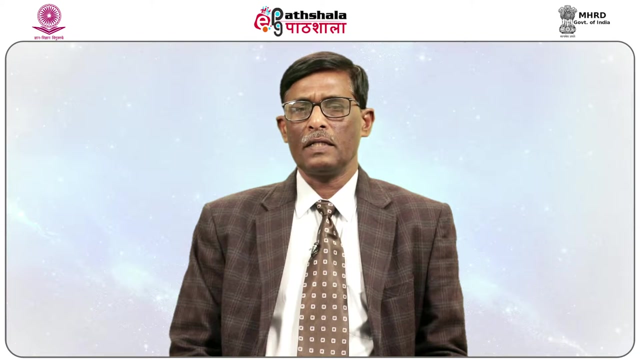 The jet stream operating in polar areas modify the weather conditions significantly because the temperature of the air is not in the best condition for the jet to transfer its energy. Therefore it does not have a good energy efficiency. The jet climate is relatively low In the case of tropical and temperate regions. the federal climate Thailandなswears a base. in the polar regions. in terms of tropical climate, The jet stream is a lower altitude and lower velocity. that is about 130 kilometer per hour During a spring and summer season. polar jet transfers energy to atmosphere effectively. Popularly known as Westerly Jet operates in subtropical and temperate regions. The normal speed of subtropical jet stream ranges from 30 to 90 kilometers per hour. The top of the jet stream is about 2.5 kilometers per hour. The top of the jet stream is about 20 kilometers per hour. The top of the jet stream is about 2.5 kilometers per hour. ranges between 160 to 190 km per hour. It significantly improves the weather conditions during winter and spring seasons in the region. The shift of subtropical jet results in improving the prospects of monsoon in tropics. Sterling jet: These winds operate in tropical zones at the speed of about 190 to 220 km. per hour. Sterling jet operate over a relatively higher altitude and also cover a larger aerial extent as compared to subtropical and polar jets. They are significant in causing descent of easterly winds near subtropics during winter and southwesterly monsoon winds near intertropical convergence zone during summer. 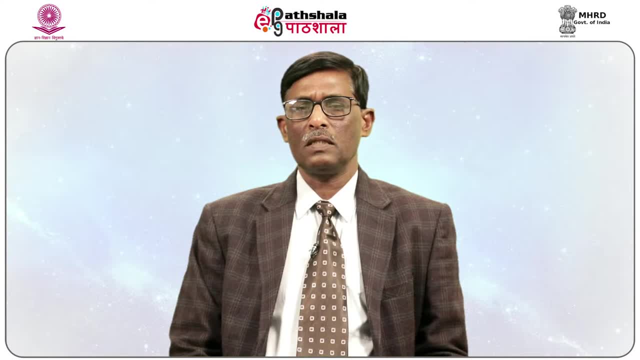 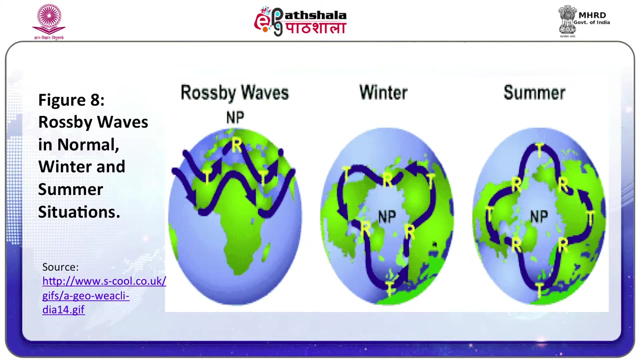 As a consequence, high pressure conditions develop in oceanic zones, in tropics. It results an increase in temperature and humidity In improving the status of southwest monsoon. let us discuss about the Roseby waves. In 1939, C G Roseby, a Swedish meteorologist, suggested that upper easterly winds in the 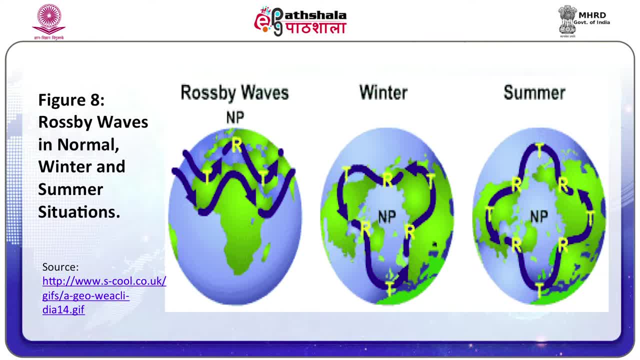 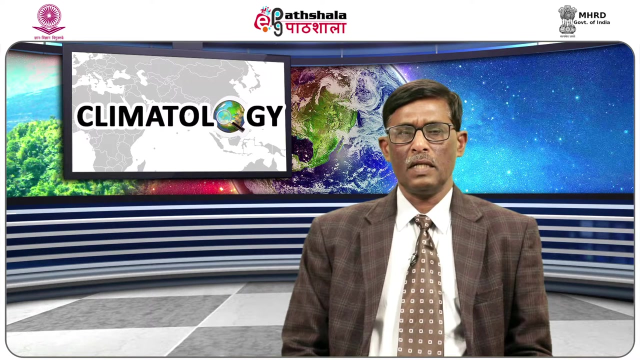 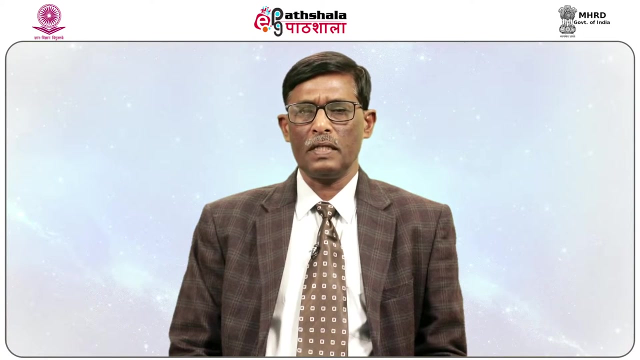 middle cell are wiped out by frictional drag and exerted by upper westerly winds. In the wall, the начина � f e d u nd tor t y w n C where are subset of inertial waves. On the Earth's these waves are giant meanders in the high 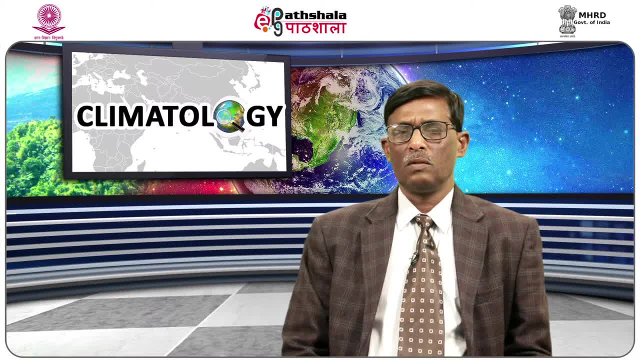 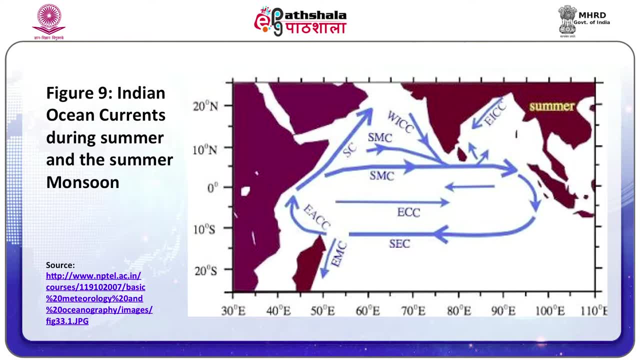 altitude winds that exercise major influence on the weather. Now let us discuss briefly about ocean waves and currents. Oscillating waves continuously transfer moisture and salt particles to the atmosphere. Similarly, ocean currents transfer water, heat and large quantities of marine biological products from equator to poles. 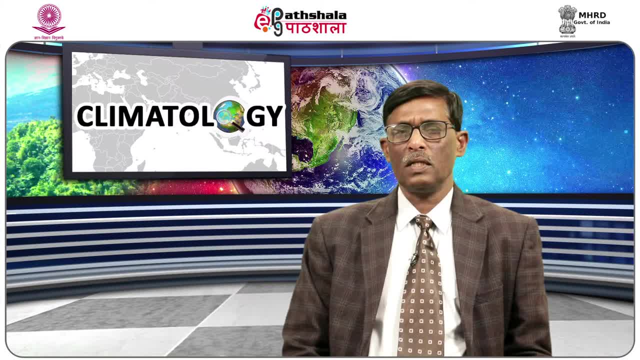 and poles to equator. In the process, ocean atmosphere maintain balance in the exchange of heat, energy and water. For example, ocean currents in Indian Ocean flow from west to east during summer, strengthening southwest summer monsoon. Thus prospects of rain increase significantly during summer. 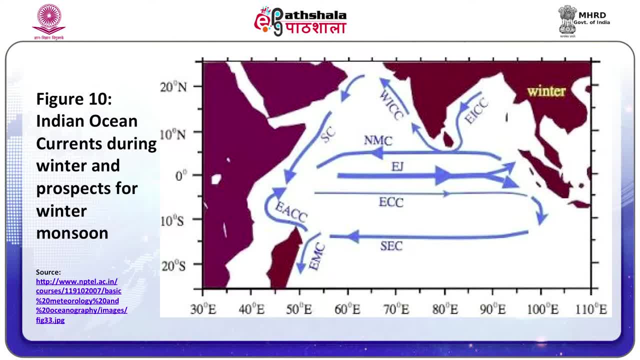 On the contrary, ocean currents in Indian Ocean flow from east to west during summer, While theмотрите ТАМИН g durasi on the hacipt of над train c, An ocean currentsンs in the eastern coast of India coincide with the direction of north-east. 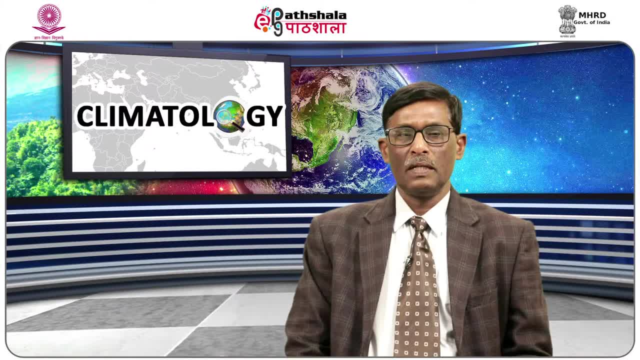 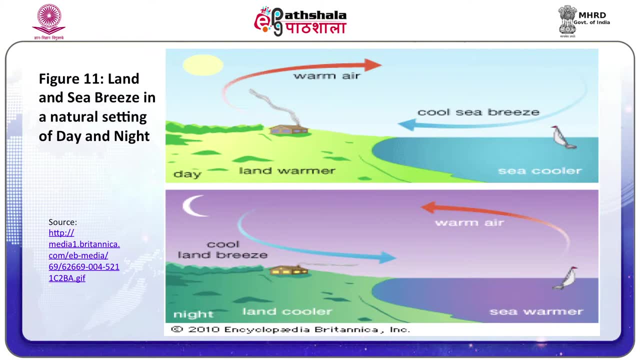 trade winds. As a consequence, TAMD region and its vicinity record sufficient rain during winter season, while t? t remains dry during summer season. Now let us discuss the деламия на land and sea songs. shirts reproduced on These are location specific bridge systems. They blow from sea to land during daytime. 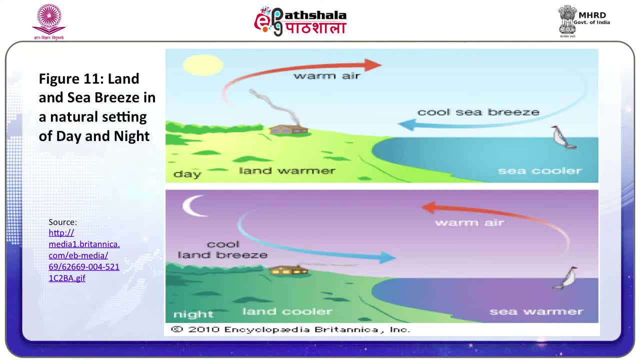 as land area gets heated quickly due to solar radiation and develops low pressure. Sea surface, on the contrary, records high air pressure during the daytime because of its slow heating process. As a consequence, wind blow from sea to land and are known as sea bridge During. 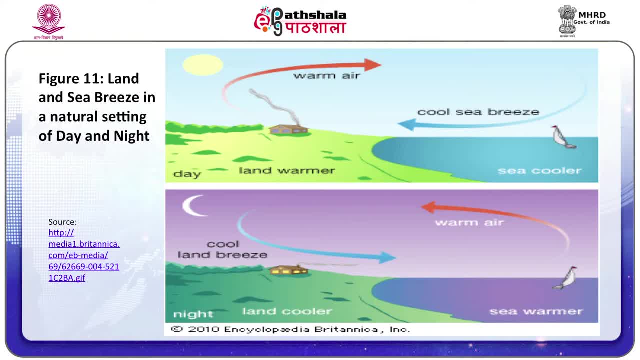 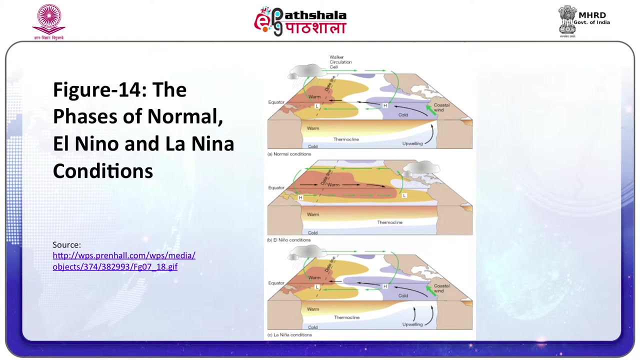 night, land area loss heat quickly and develops a high pressure, whereas sea surface remains comparatively warmer and thus develop a low air pressure. As a consequence, winds blow from land to sea during night and are known as land bridge. Now coming to L-nino phases, Ocean atmosphere interaction is studied in terms of occurrence. 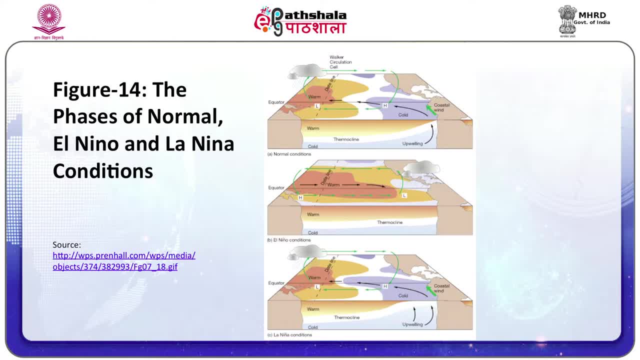 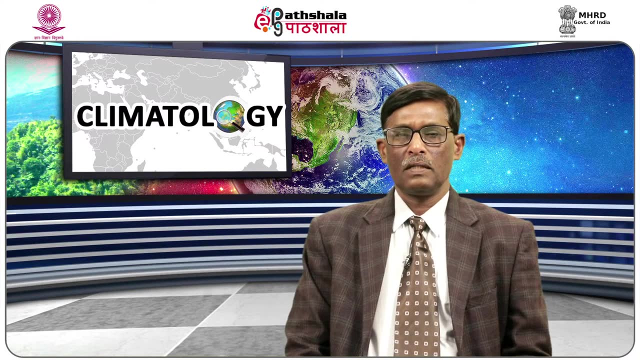 of L-nino and southern oscillation. The two concepts have been put together to be known as ENSO. There are two basic concepts related to ENSO phenomena. These are sea surface temperature, that is SST, and sea level pressure, that is SLP. 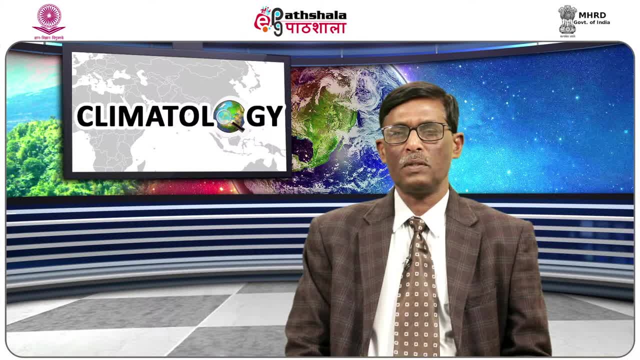 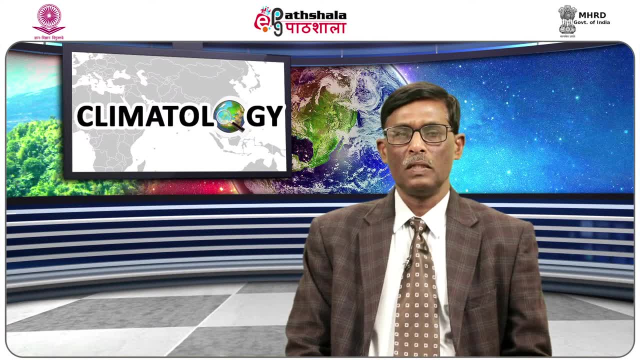 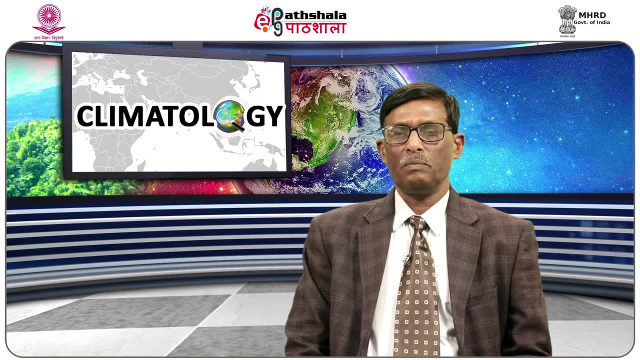 The term El Nino refers to the extended episodes of anomalous warming of the ocean of the coast of Peru. The term Southern Oscillation refers to a sea level pressure swing between Darwin Island, near Australia, and the island of Tahiti in central tropical Pacific. 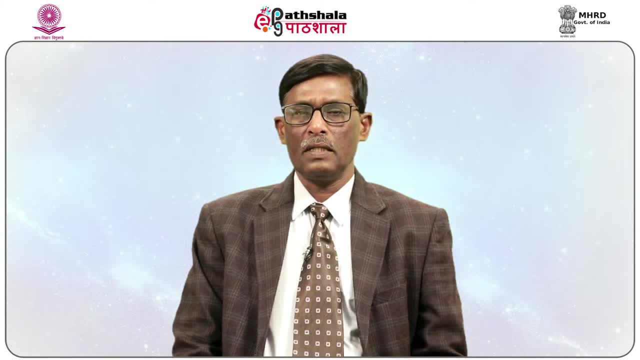 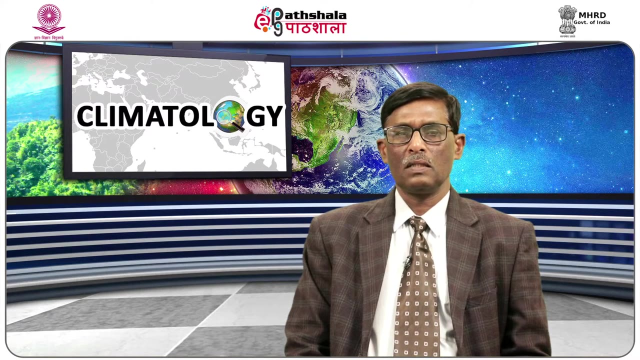 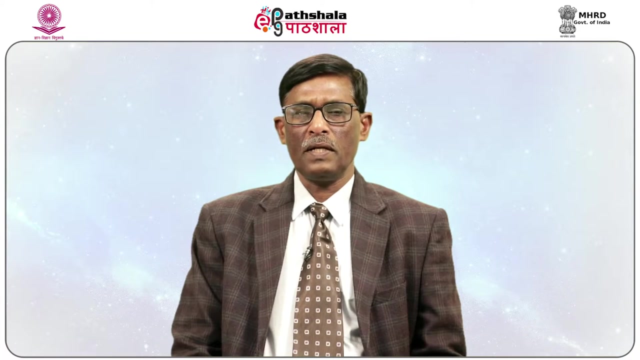 Jerkins in 1969 recognized that El Nino and the Southern Oscillation that is ENSO are in fact just two different aspects of the ocean. Ocean-atmosphere interaction is at the heart of the ENSO phenomenon. An initial change in the ocean could affect the atmosphere in such a manner that the altered 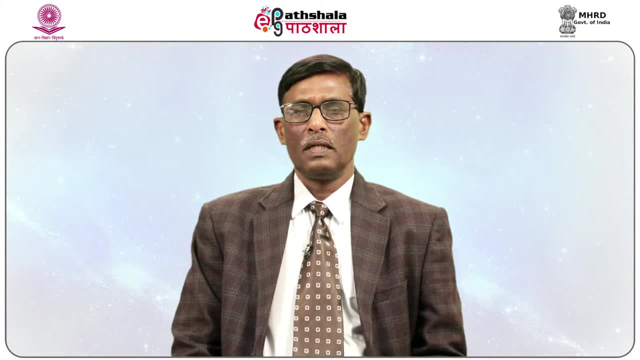 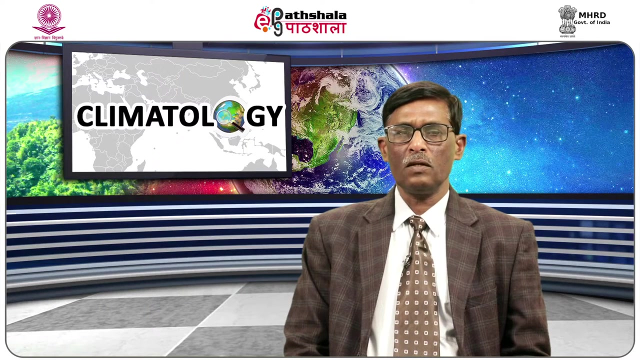 atmospheric conditions would in turn induce oceanic changes that reinforce the initial change. The atmosphere will respond by reducing the atmospheric pressure of the ocean. Theization of photosynthesis means reducing the functional pressure of the ocean at Lovely altitude. This is follow up, the And now. the info may not be immediately. Nothing will be yet. Caffeta. I am Sonali J pet legit yet added 15 books by Christian Watters and Yang Shi-jiebie. There is a tillage offshore once to demonstrate the classes of to lowest, and thì in this case, something is not exactly the last time direction. rather, we have to see how the altitude can. 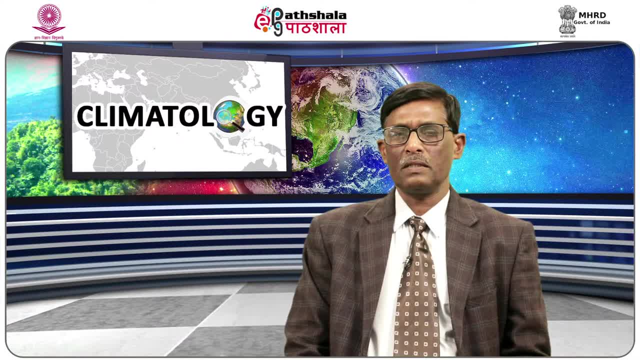 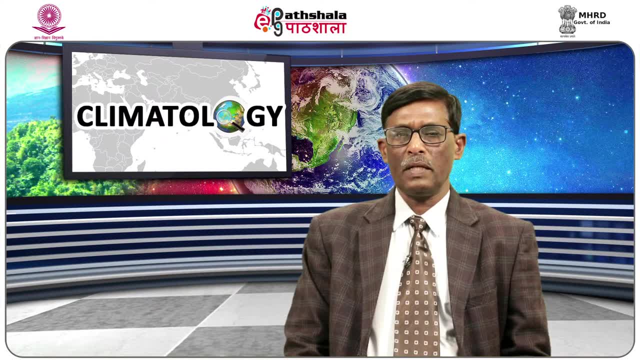 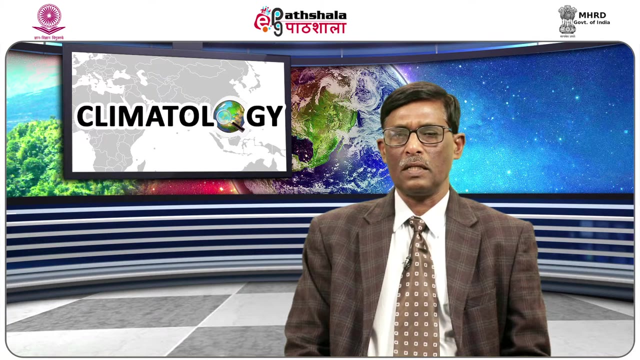 small initial perturbations into large observable amplitudes. The satellite-based observations have played an important role in understanding ARC interaction and climate research, particularly in outgoing long-wave radiations and SST. Space-borne microwave sensors have enabled all weather observations of SST rainfall. 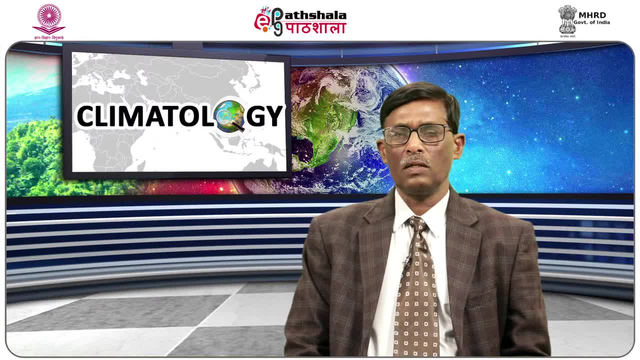 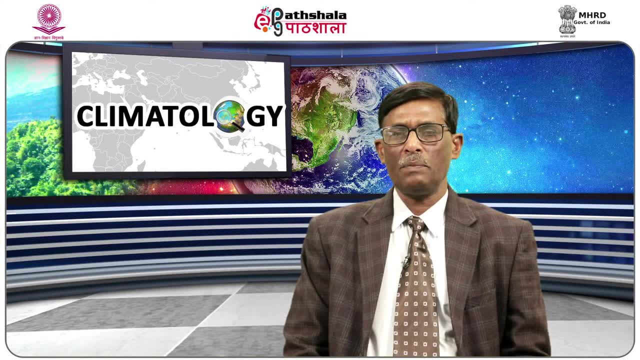 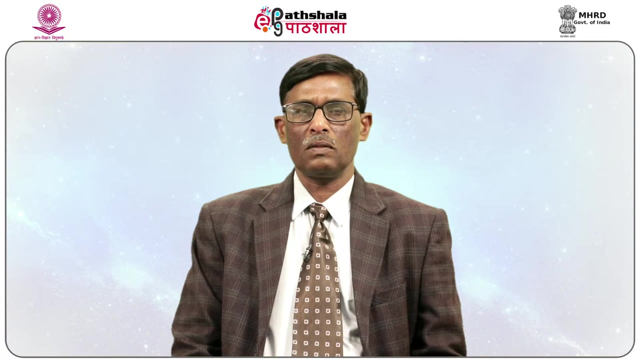 surface wind and ocean surface height over the global ocean. With such a database, there has been rapid progress in understanding and simulating the climate and its variations. Jerkins, Manaves and Bacchus Brand were the first to work on ocean atmosphere general circulation model. 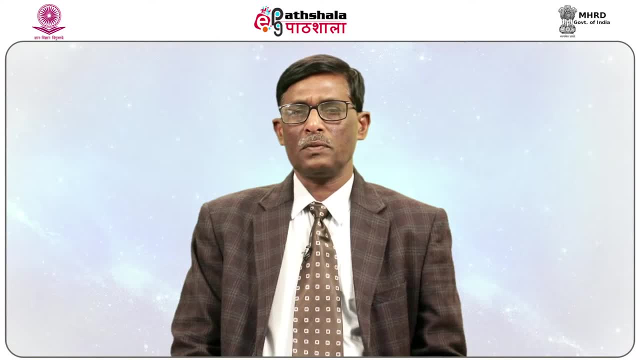 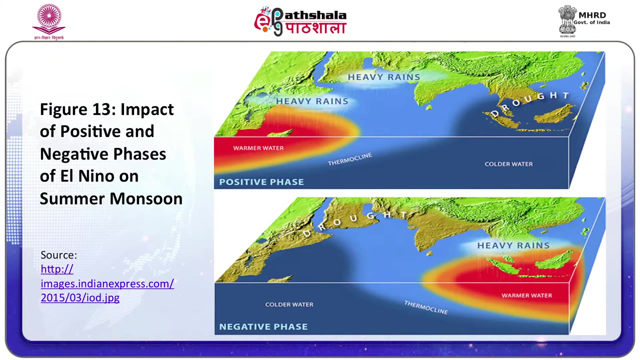 Since then, occupied ocean atmosphere models are being used to work out interaction for ocean atmosphere circulation. Coming to El Nino and Monsoon. The term El Nino refers to the extended episodes of anomalous warming of the ocean atmosphere In the past. you may have seen the 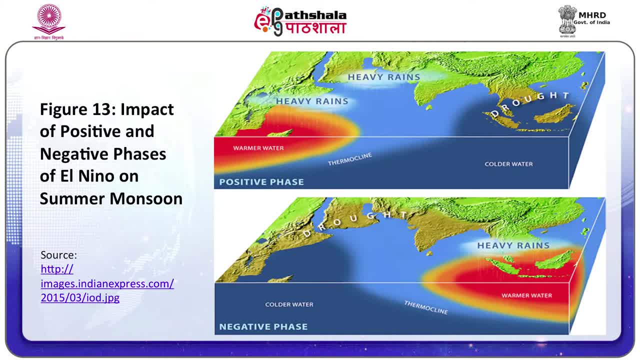 El Nino hurricane breaking into the Pacific Ocean in the late 1970s. In the 1980s, it was a tidal wave that caused the Earth's surface to cause佔odate With this, the current population of the coast of Peru. on specific years when the sea surface. 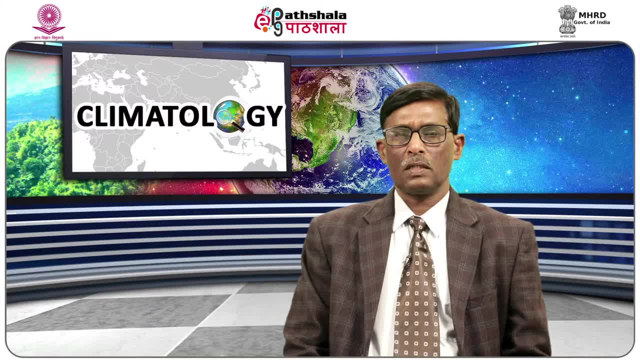 temperatures in the equatorial Eastern Pacific are enormously warm. the east-west gradient in SST will be reduced. It results in the wakening of monsoon. The effect of El Nino on summer monsoon is significant. El Nino is a warm ocean current. 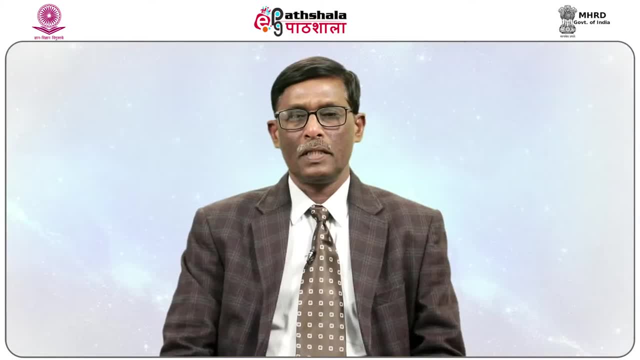 It will continue to cause a condensate in El Nino to the west west and to the east east, But it will happen. It will happen, appearing along the coast of Peru. The appearance of El Nino reverts the condition of Peru current. 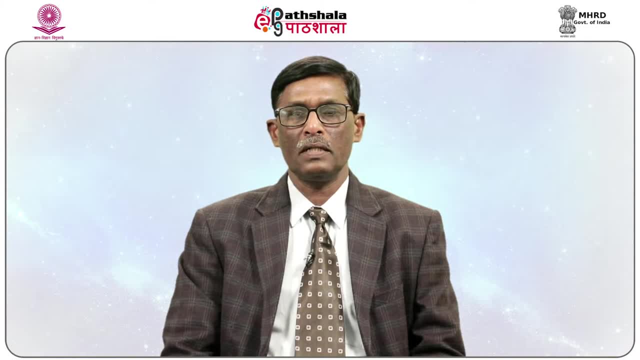 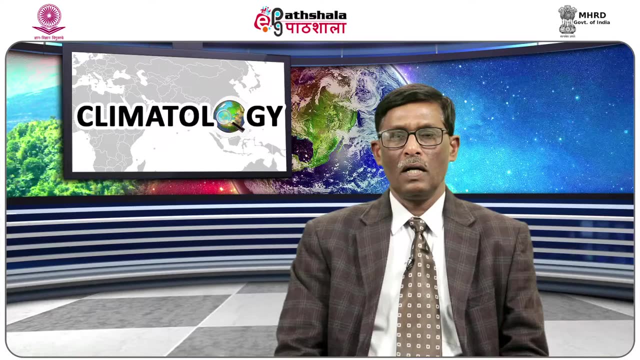 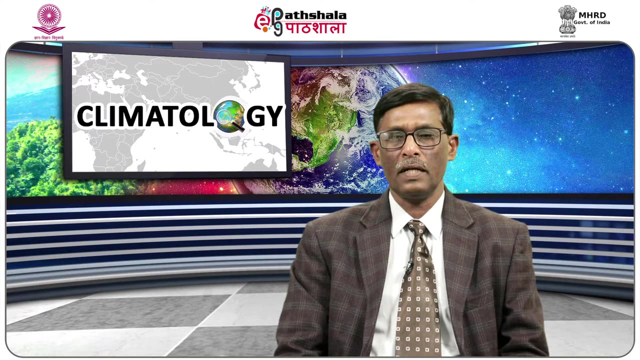 by developing warm water and moist air conditions over Eastern Pacific and cold conditions in Western Pacific. As a result, Eastern Pacific along Peruvian coast in South America records high rainfall, while Western Pacific along Australian and Indonesian coast record drought conditions. El Nino results in weakening of the monsoon, causing drought conditions. 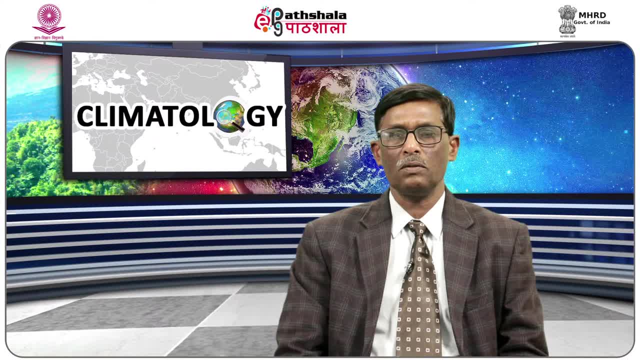 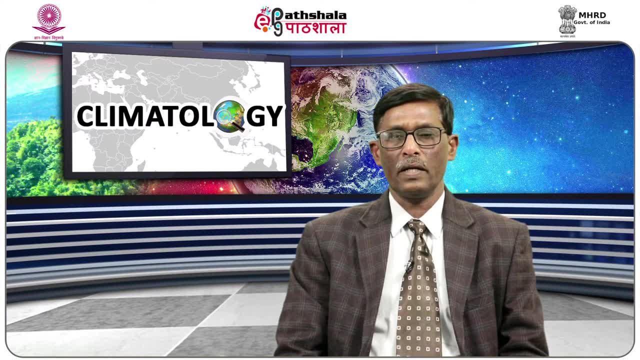 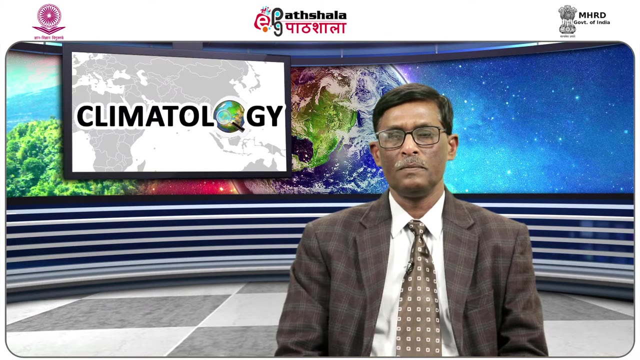 and crop failure in monsoon regions of South and Southeast Asia. When Western Indian Ocean records low air pressure during winter and high air pressure during summer, it is said to be the positive phase of summer. monsoon and sea surface conditions are normal. Heavy rains are caused. 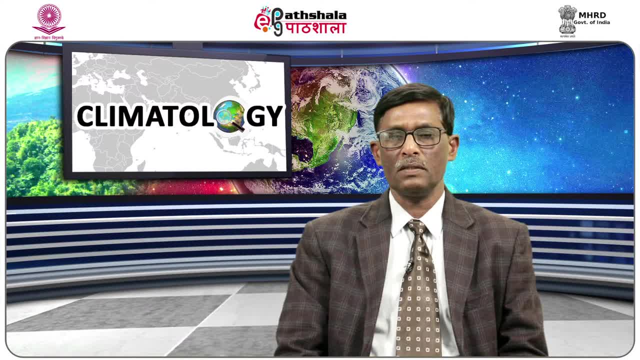 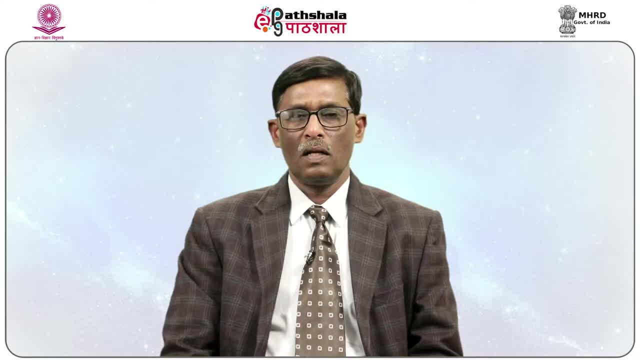 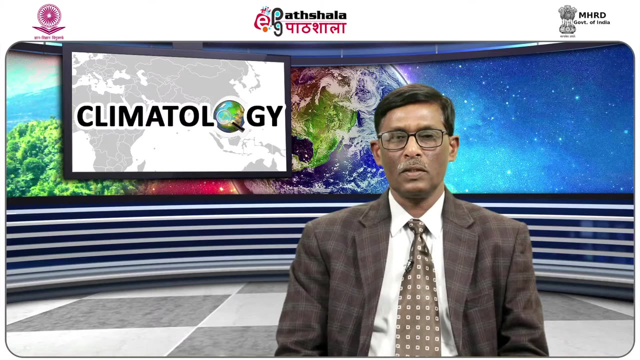 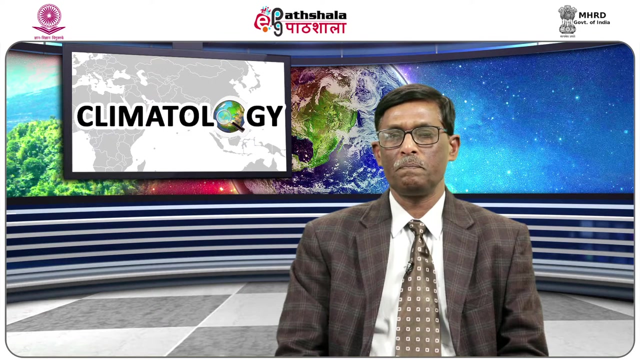 in Indian subcontinent and neighboring regions during normal phase. Now coming to the La Nina and monsoon relationship. La Nina- the word originates from Spanish, meaning little girl. It is characterized by usually cold ocean temperatures in Equatorial Pacific. During the period of La Nina, the sea surface temperature across Equatorial Central Pacific Ocean becomes. 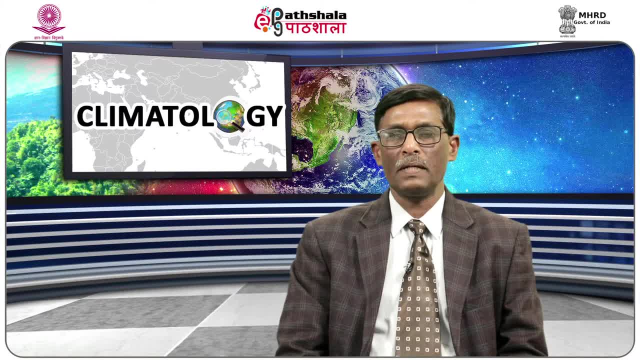 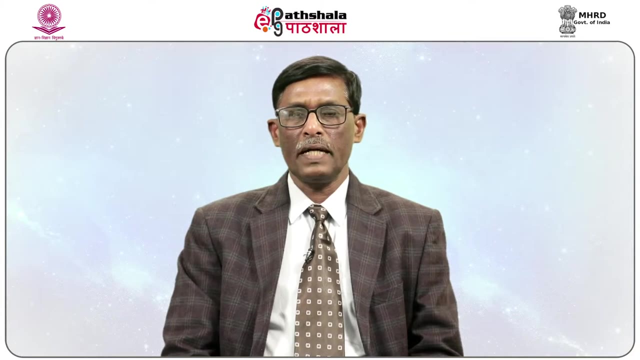 lower than normal by 3 to 5 degrees Celsius. It has extensive effect on the weather in North America, even affecting Atlantic hurricane. La Nina causes heavy rains over Malaysia and Philippines and Indonesia. Western side of the Equatorial Pacific is characterized by warm, wet, low pressure weather. 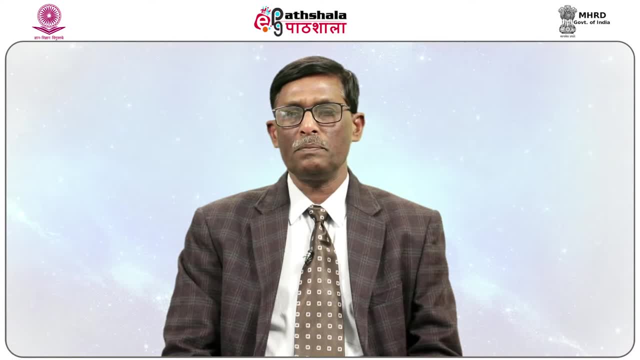 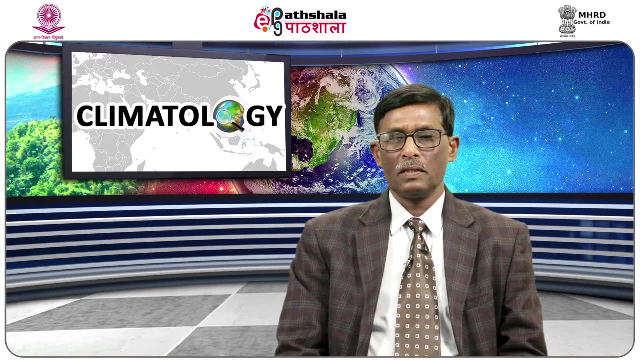 as the collected moisture is dumped in the form of typhoons and thunderstorms. As a result of this, the surface water of the Western Pacific is 60 cm higher compared to the western Pacific coast. Now coming to the Southern Oscillation Phases. Southern Oscillation is linked to low frequency. 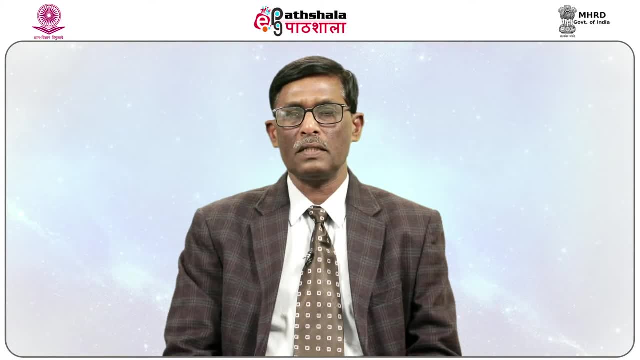 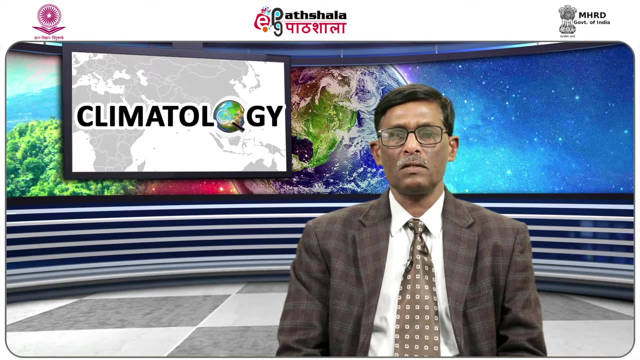 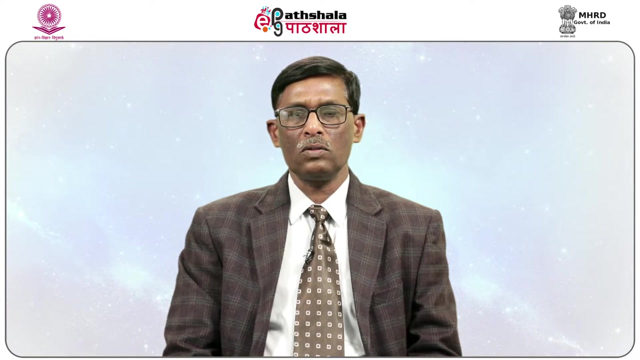 temporal fluctuations in sea surface temperature in the Equatorial Pacific Ocean. It is one of a number of many, many manifestations of atmospheric fluctuations associated with alternating episodes of warm and cool sea surface temperature in the equatorial Pacific Ocean. Its impact are also experienced in Indian Ocean, where it influences the mechanism of monsoon. If air pressure along equatorial 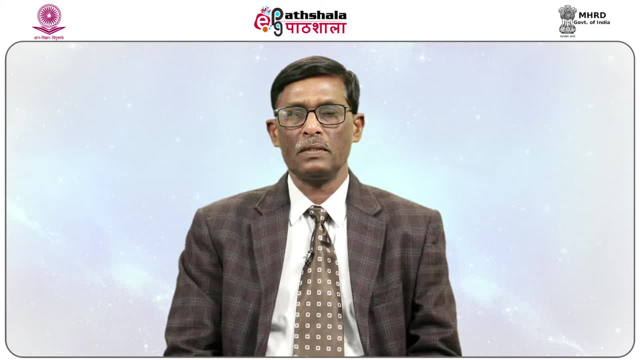 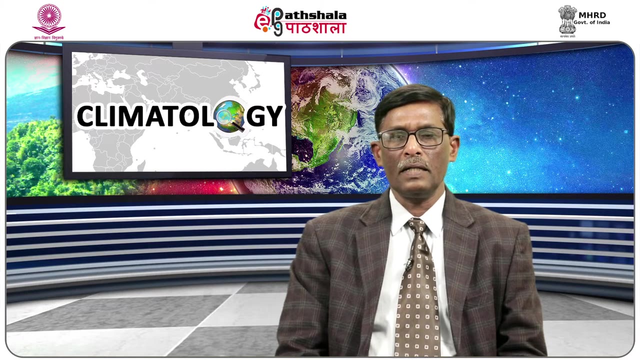 Pacific Ocean is higher than the air pressure in the Indian Ocean during winter, it is said to be a positive southern oscillation, indicating a favorable monsoon. When air pressure during winter is higher in Indian Ocean and lower in Pacific Ocean, it is known as negative southern oscillation. 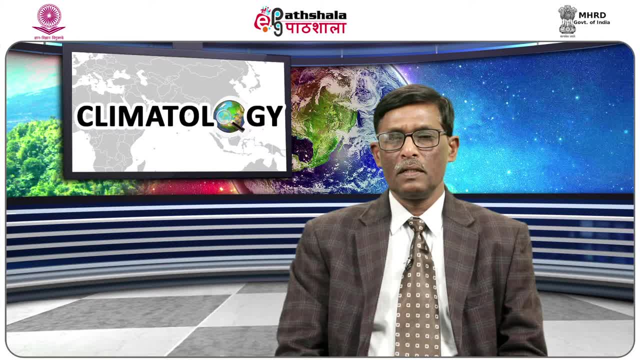 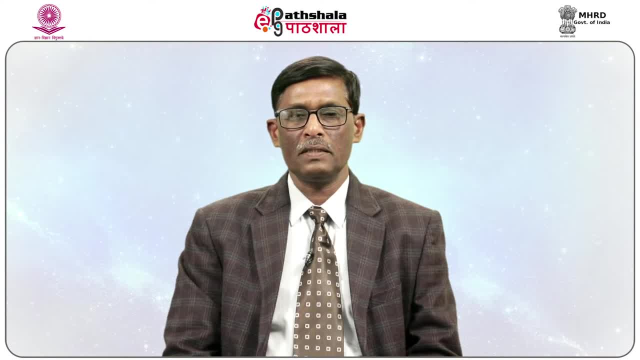 Such a situation results in a weakening of summer monsoon. The intensity of southern oscillations is worked out by the difference in sea level air pressure at Tahiti, which is situated at around 18 degree south, and 149 degree west longitude, A station in mid-Pacific, and Port Darwin, which is situated at 12 degree. 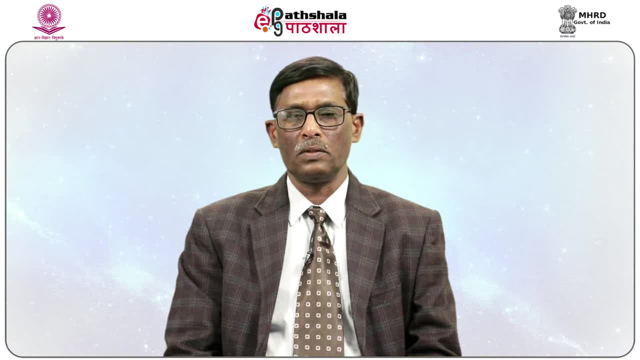 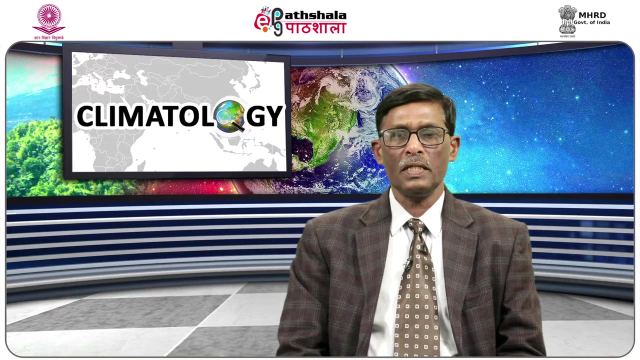 south latitude and 130 degree east longitude, a representative station in the Indian Ocean. A negative value of southern oscillation index implies low pressure over the Peru coast and high pressure over the Indian Ocean during winter season, explaining a poor monsoon phasesSo there seems to be a close correlation between the appearance of air liquid and ran. 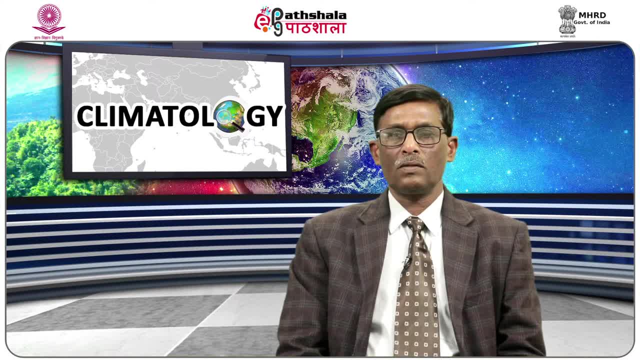 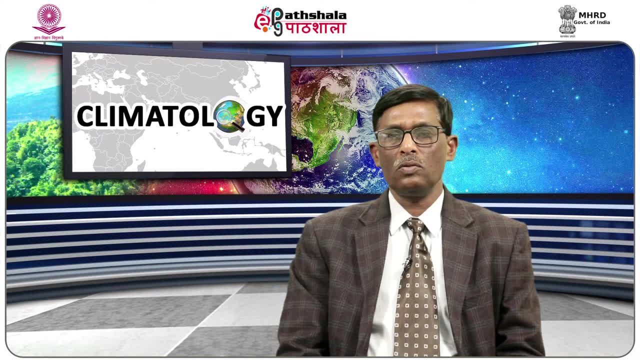 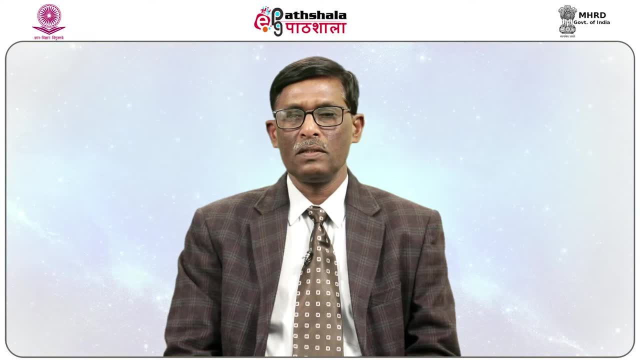 Nino and the negative SOI Southern Oscillation has a period ranging between 2 to 7 years. Now coming to the positive Southern Oscillation, It has been established that when sea level surface pressure is high over the Pacific, air pressure over Indian Ocean tends to be. 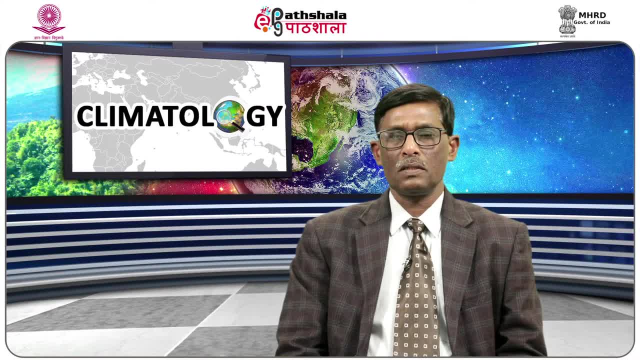 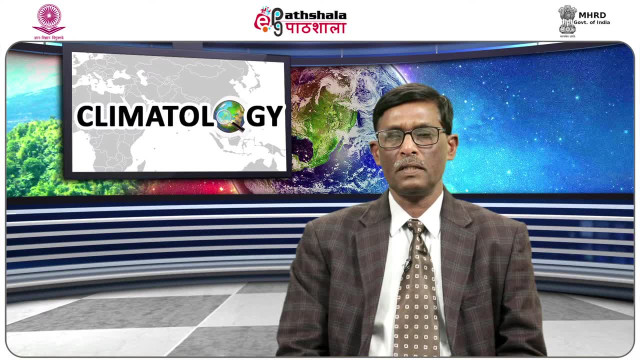 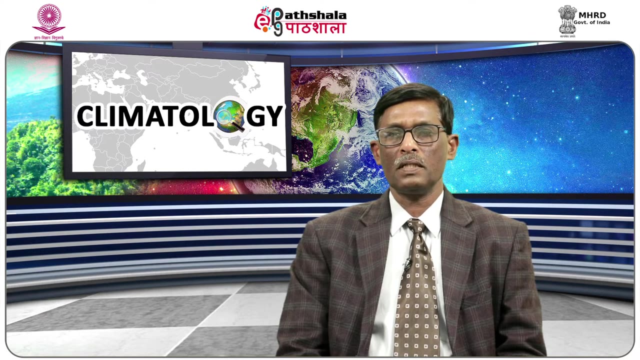 low. Since surface air pressure over oceans during winter season is inversely related to summer rainfall, prevalence of low air pressure over Indian Ocean during winter season is considered to be a sign of positive Southern Oscillation. The chance of favorable monsoon are generally linked with positive Southern Oscillation. 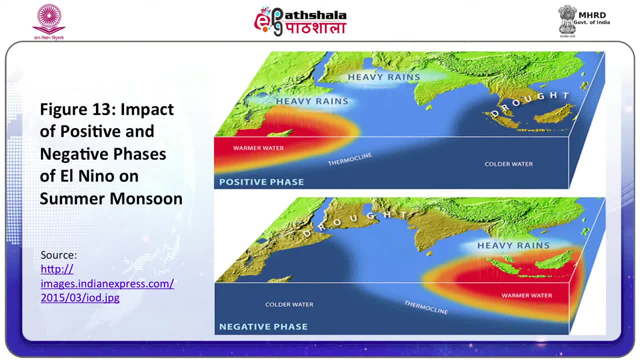 Now coming to the negative Southern Oscillation. The prevalence of high sea level pressure over Indian Ocean and low air pressure over Pacific Ocean during winter denotes the negative Southern Oscillation. It has been established that negative Southern Oscillation index is linked with a weak monsoon phase. 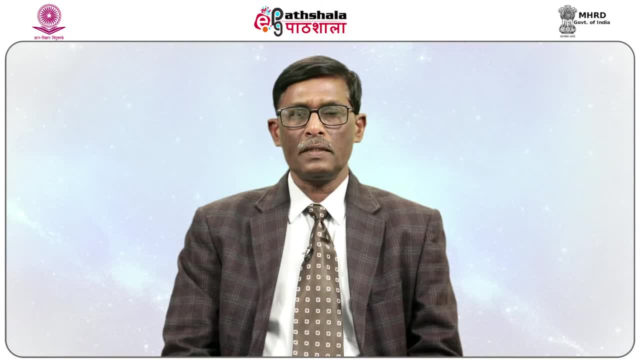 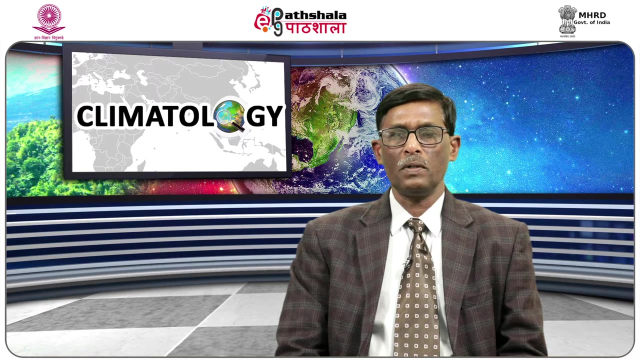 Now coming to the seasonal cycle, Solar radiation is dominating the Earth's atmosphere. It is illuminated in H to the south and international horizons to the east and west. In the central hemisphere, solar radiation is illuminated in X direction and Y direction. Solar radiation is usually transmitted from 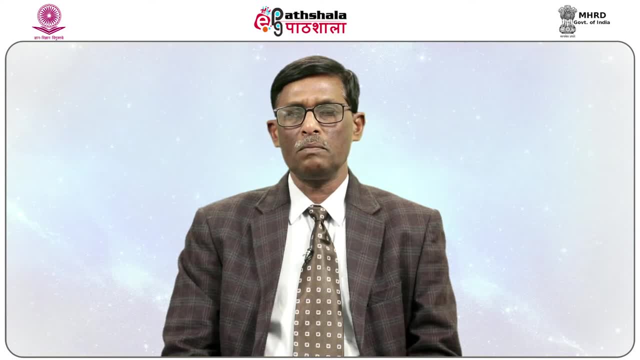 the opposite side of the earth, to the east and south of the earth, The Florence indicator is illuminated by H, determined by the calendar of Earth's observable atmosphere. This rescued the Earth by the velocity of itsから Planck. These are isolated by a single wave, For example. 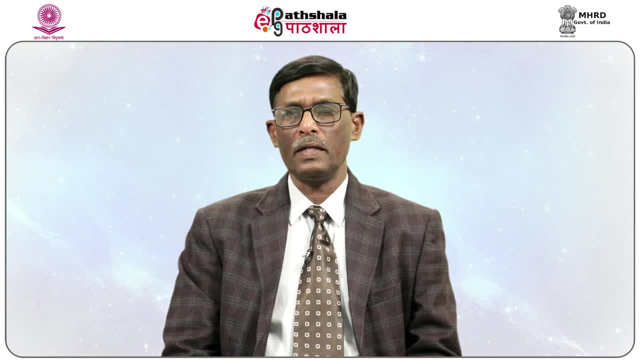 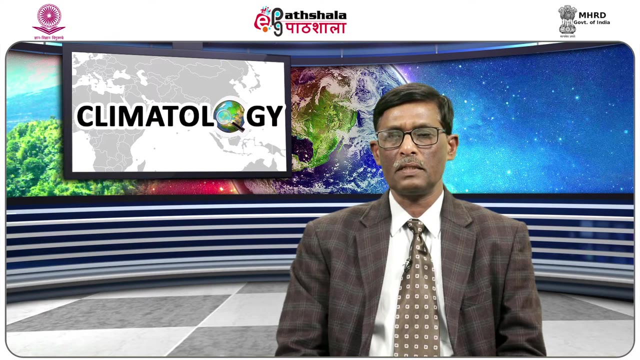 after 3 months from summer and winter solstice. It is mainly due to a lag in large thermal inertia of the upper ocean. This local waxing and waning of solar radiation is a reliable predictor of season over most of the world except on the equator. The annual harmonic 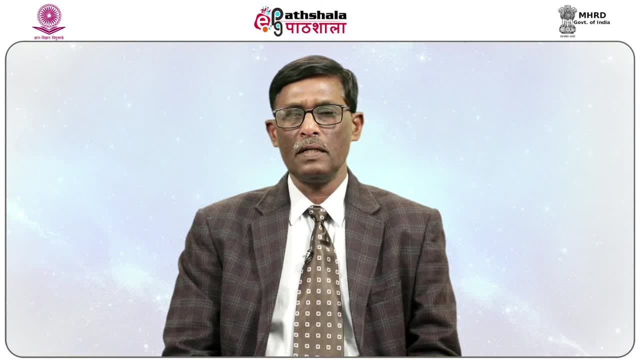 of solar radiation reaches a minimum near the equator. The same time, the pronounced annual cycle in SST is also observed in the Eastern Pacific and Atlantic Ocean. The climatological mean thermocline is shallow on both the locations. For example, the annual range of SST near 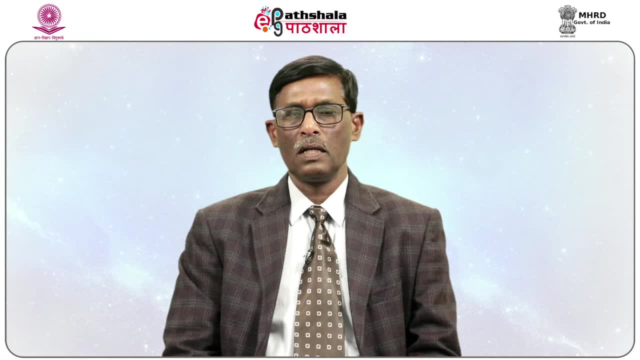 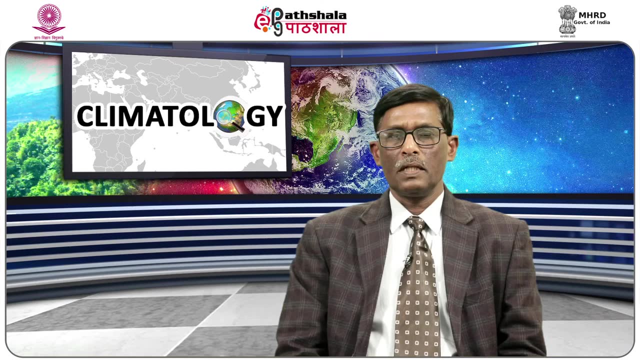 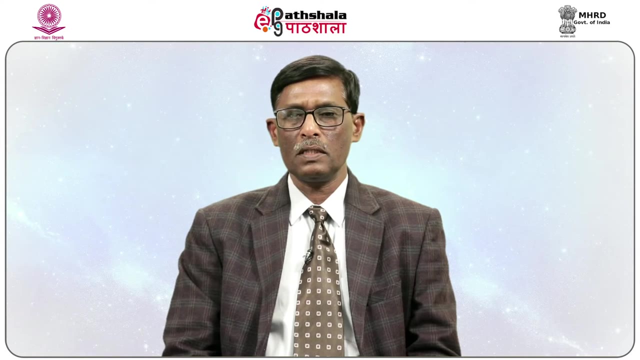 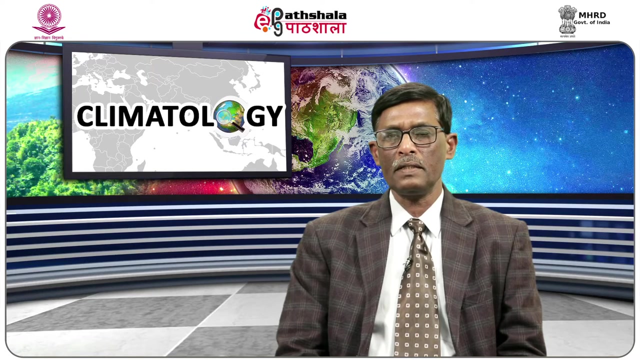 the Galapagos Islands is about 6°C greater than most of the tropical oceans. It is to be noted that there is a westward co-propagation of seasonal SST and zonal wind anomalies along the equator in the Eastern Pacatic, Significant increase from normal temperature in winters. 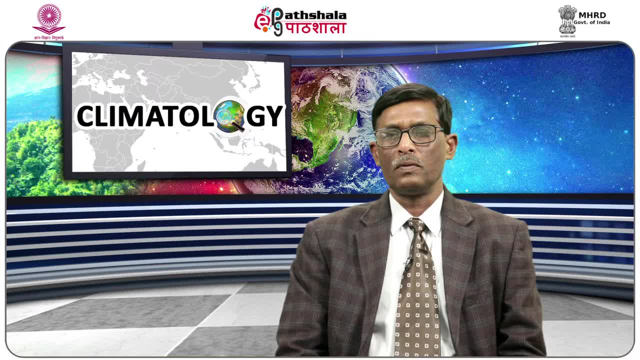 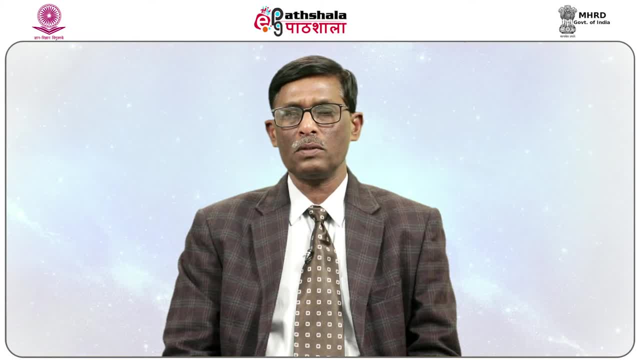 explains the occurrence fact As much as the zone nativity properties is the same on the of El Nino. Now let us conclude this module. Solar heating is the basis for ocean-atmosphere interaction. The motions of the earth with reference to sun are responsible for the generation. 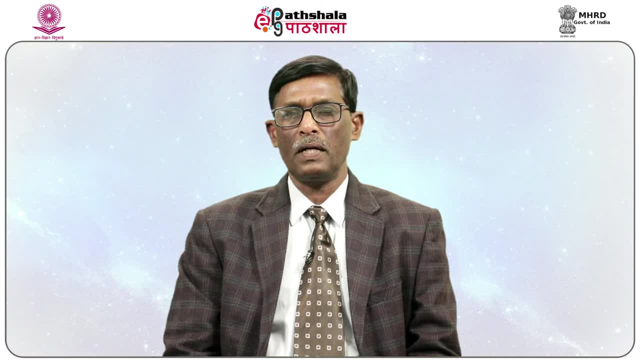 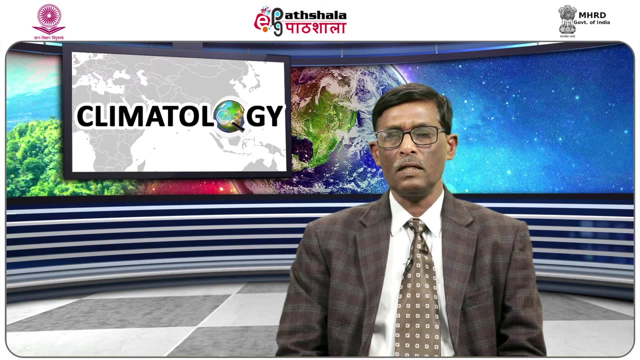 of energy and its distribution in different parts of the earth. The earth's rotation results in causing day and night. The cycle of interaction is augmented by processes such as radiation conduction and convection. The energy so transferred is subjected to modification by the process.